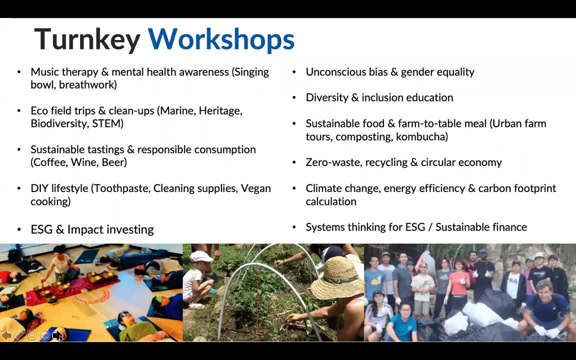 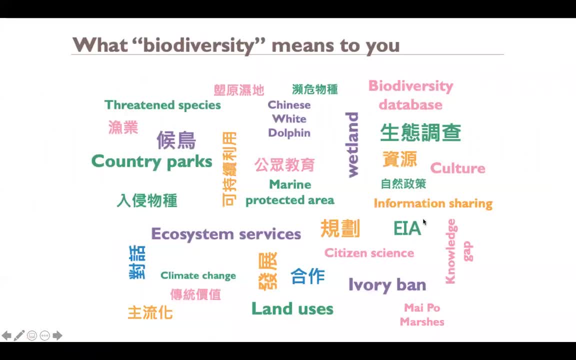 So welcome to our website to learn more If you want to after this talk. you're interested. So I'm going to start with biodiversity. What's the definition? And you're welcome to put it in your chat If you want to try this answer. 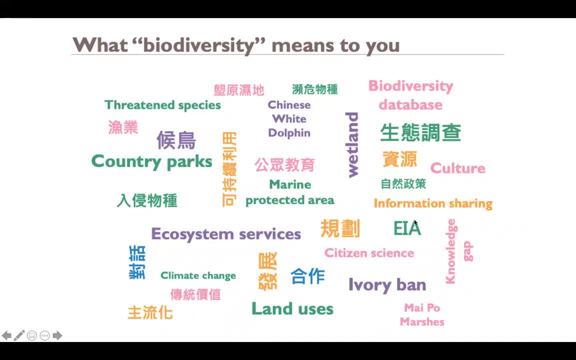 I don't know. what does biodiversity mean for you When you think about this? what do we mean? So anybody want to try. It's not that easy. actually, It's not a very straightforward answer. So biodiversity means three things. It means the genetic diversity. 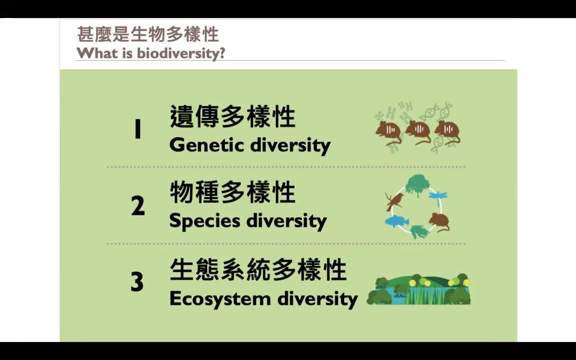 For example, within the species, if they're really diverse enough. It also means species diversity, which is number of species there, which is like what we usually think of when we talk about species, And it also talks about ecosystem diversity. Today is there a different habitat where animals can live. 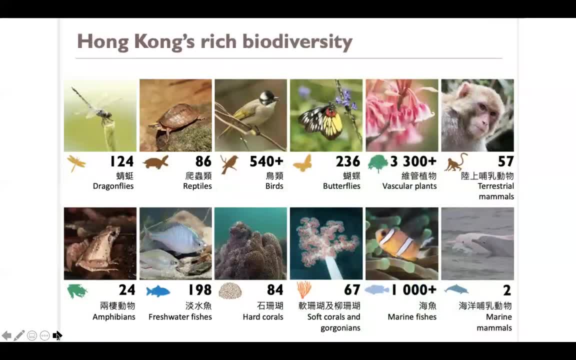 So in Hong Kong- this is a snapshot, This is from the AFCD. So we have over a thousand number of marine fishes. We also have marine animals like Chinese white dolphin. You might know We also have a number of soft coral and gorgonian. 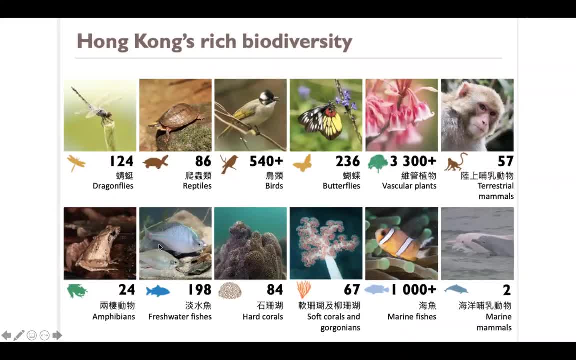 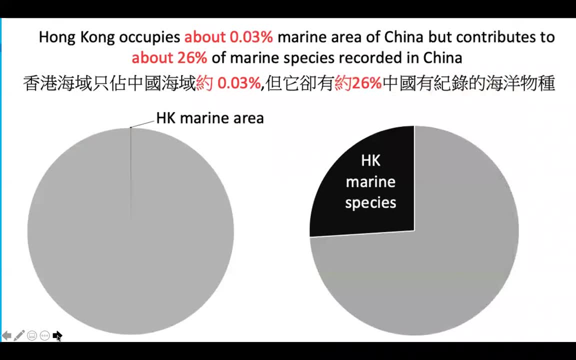 We have 84 species of hard corals and then we have fish and all that. So we are quite not bad in Hong Kong. So another case in point is Hong Kong. We only have 0.3% of all the marine area in China. 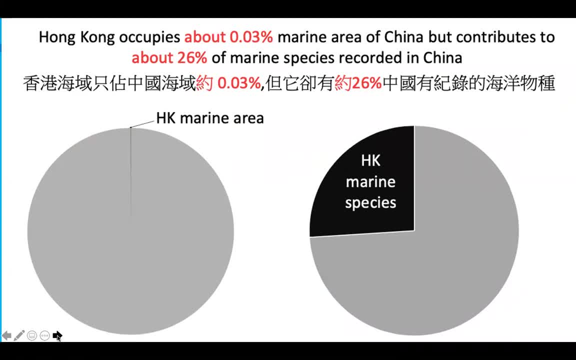 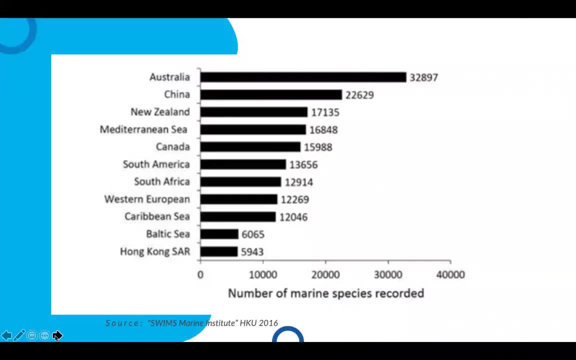 but we actually have over 26% of the species that are recorded in China. So this is just showing you how diverse we are as a habitat, And we are actually comparable to Caribbean Sea. So, for example, in Caribbean there's 64 species of coral. 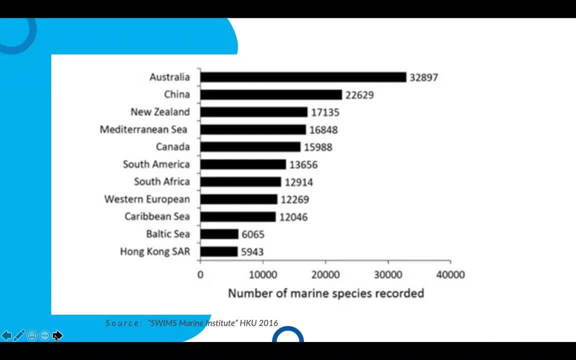 In Hong Kong we have 84 species of hard coral, So in terms of coral, we are actually better than in Caribbean. So even though Hong Kong is just a small area, we are actually not bad. So there's always a lot of people asking me whether it's good to dive in Hong Kong. 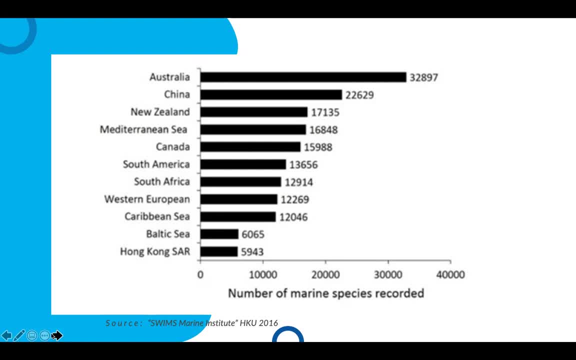 So my answer is: Hong Kong doesn't have the perfect visibility, It's not Bali, It's not Indonesia, It's not Kota Kinabalu, But we do have some stuff to see, and today I'm going to share with you what those are. 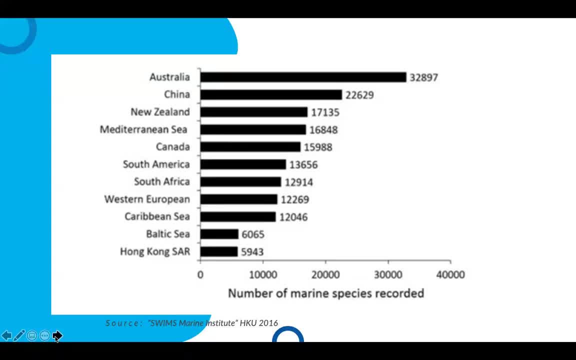 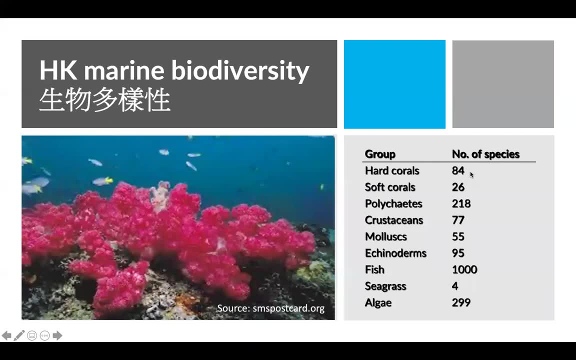 Anybody joining? Not yet. Okay, So, oops. So, as I said, Hong Kong has 84 species of hard coral. These are just numbers here, Don't worry about it, You have this slide, But I just want to show you the sheer number of species we have. 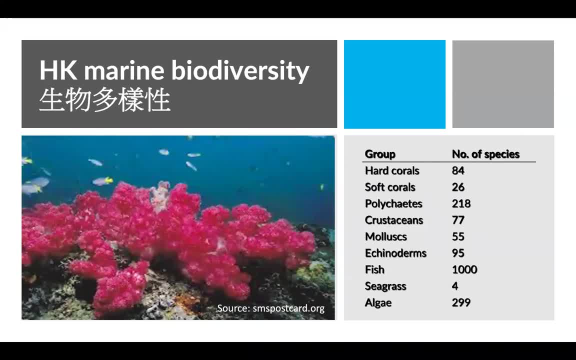 And we are discovering new species every year. For example, last year I think there was a study on redfishes. There were three new redfishes that were found in Hong Kong, So these numbers are keep rising. So in Hong Kong we have some species that are named after Hong Kong. 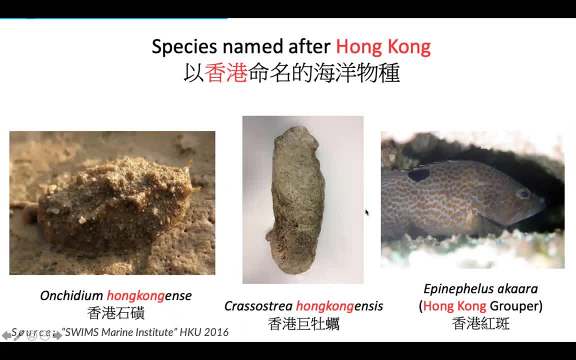 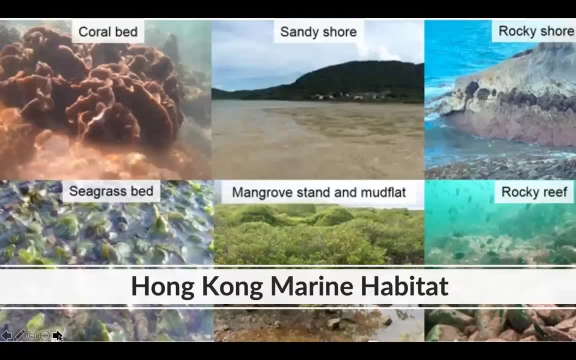 So, for example, Hong Kong grouper- for those of you enjoy seafood, you might have come across in the seafood restaurant We also have this two-walkie-shaws animal. So in Hong Kong we have different marine habitat. So today I'm going to share with you. 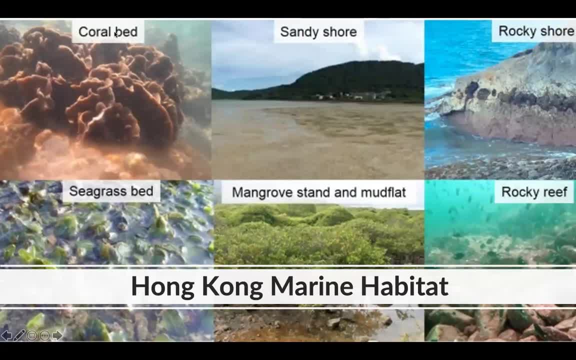 going to mostly focus on the species that we have found in the coral bed in Rocky Reef, which is most diverse. I'm going to put less emphasis on the species in Waukesha. so, just because of the interest of time, so maybe if I do, 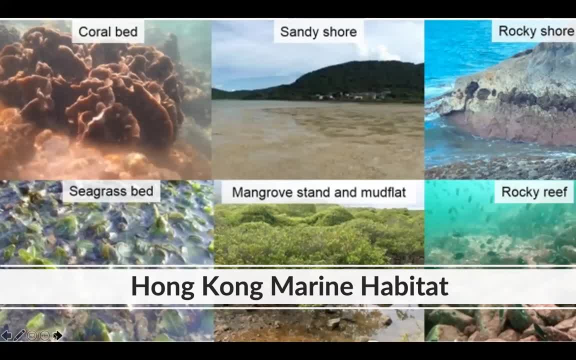 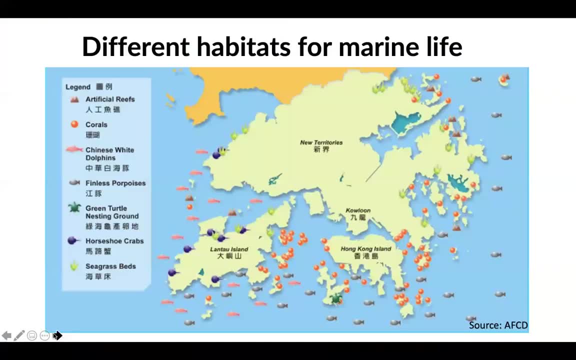 another talk. I will focus on that. But just to let you know, this is not by no means comprehensive for Hong Kong. So where can we find the animals, So the Chinese white dolphin, which a lot of various animatic species, are on the? 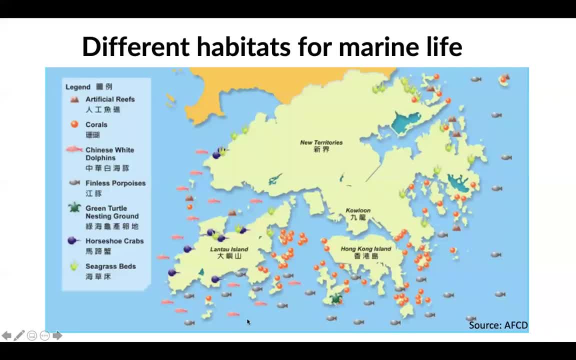 western part of the shore. the coral is usually on the eastern side, and here this green side is the Samoan. it's the special scientific site where the green turtle breed, and then we have some horseshoe crab in Lantau Island and I. 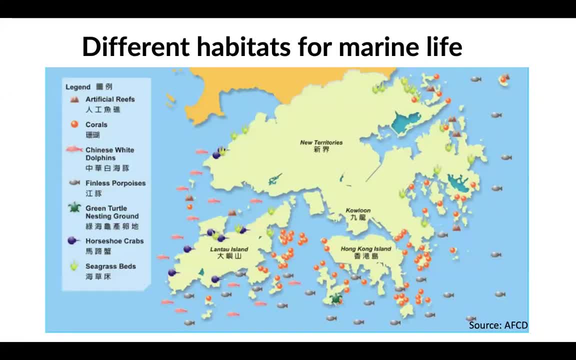 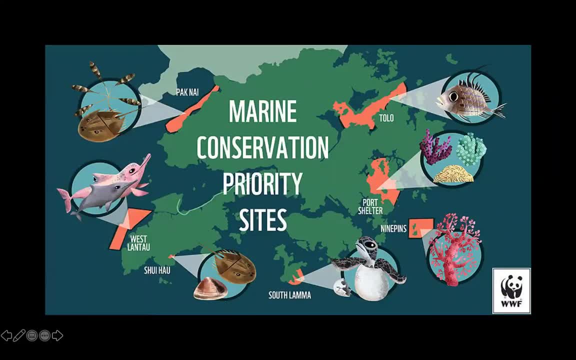 will tell you in a bit why do they live there and what challenges they face. So this is another diagram. as I said, the dolphins on the west side, horseshoe crab in here and here as well, the sea turtle, and then we have a lot of. 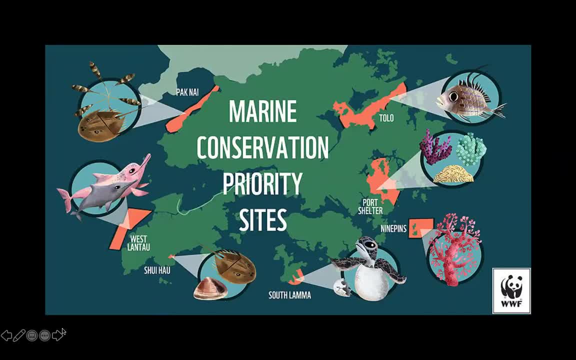 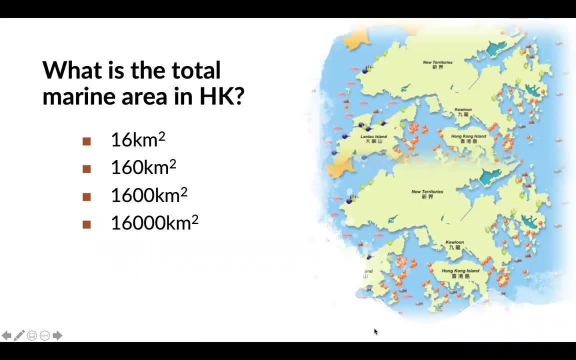 corals and in the total harbour is also good with fish. So first question, and I hope all of you can participate: do you know what is the total marine area in Hong Kong? And you can type the answer in the chat box So anybody want to try. 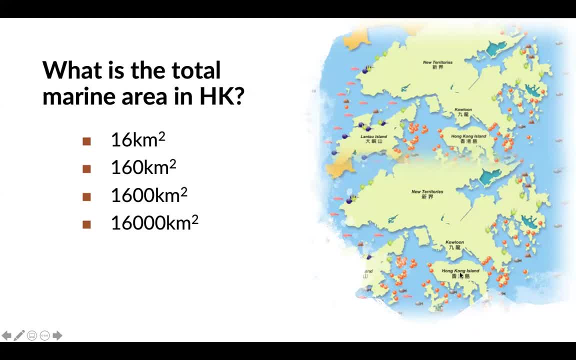 And if I give you some incentive, those who answer most correctly today will get a special prize from me. you will have a discount, Yeah, so let's see. what do you think? Okay, the answer is actually 1,600.. We have quite a. 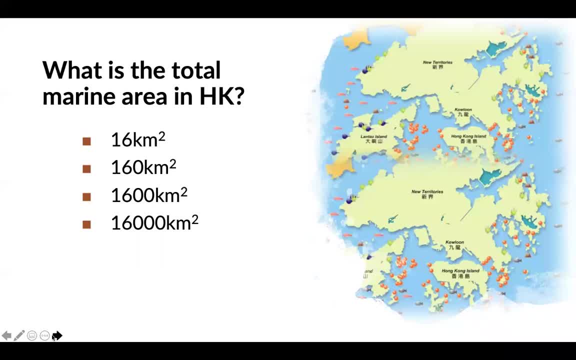 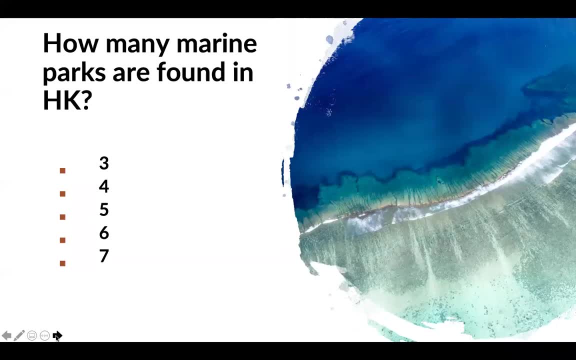 bit of marine area in Hong Kong, and what are those marine areas used for? So this is another question. so I will give you a tip. Just now I showed you a video of Hoi Ha and he said there's a certain number of marine parks in Hong Kong That 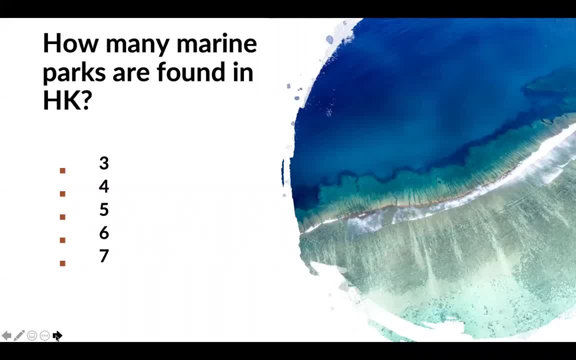 is an old video, two years ago. it's no longer updated. We have a new marine park in Hong Kong just two months ago, So can you guess how many marine parks are in Hong Kong? Anybody else want to guess other than Chim Lo? 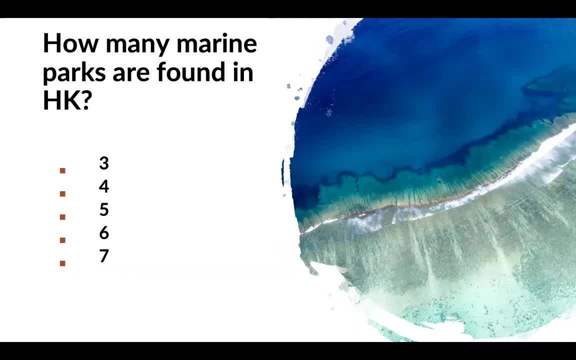 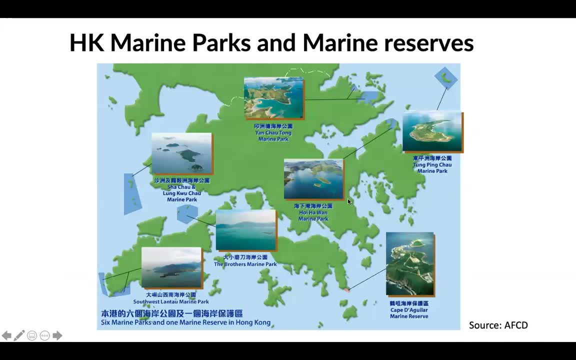 Okay, we have very different answers. Okay, the answer is six. So these three marine parks- Nhan Chau, Tong, Tong Ping Chau and Hoi Ha Wan- they are very good for coral diversity. So the number one coral diversity is in Tong Ping Chau. it has almost all of. 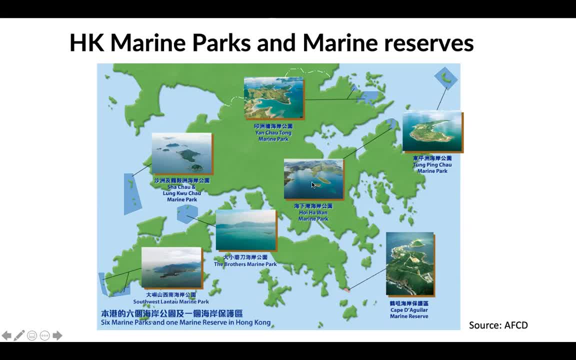 the 84 corals in Hong Kong. Hoi Ha Wan is the second. it has 64. And these three on the left hand side is for the Chinese white dolphin, And the southwest Lantau Marine Park is the newest marine park. 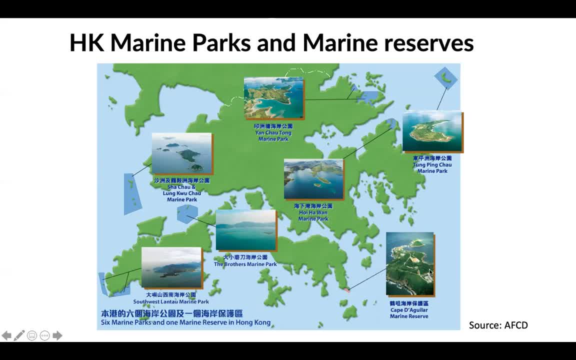 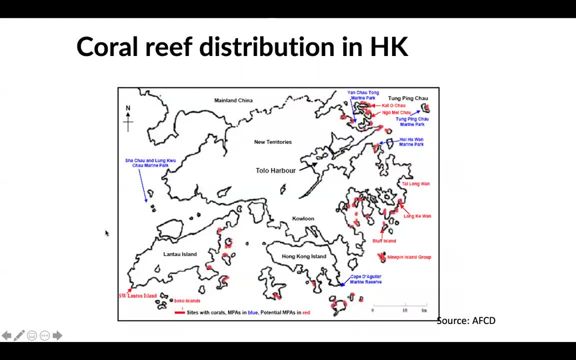 And here in Cape D'oglaura is a marine reserve, not a marine park, which is protected from its rocky reefs. So most of the coral we find in Hong Kong are on the eastern, northeastern side. Anybody know why, or anybody want to guess why, that? 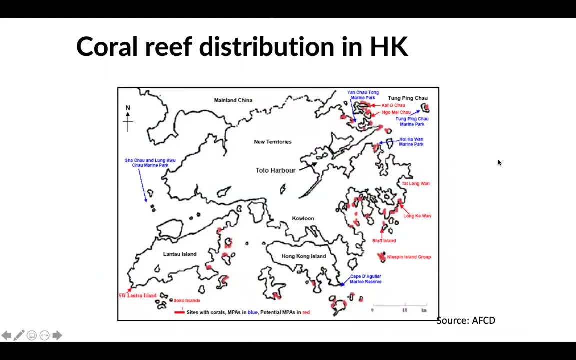 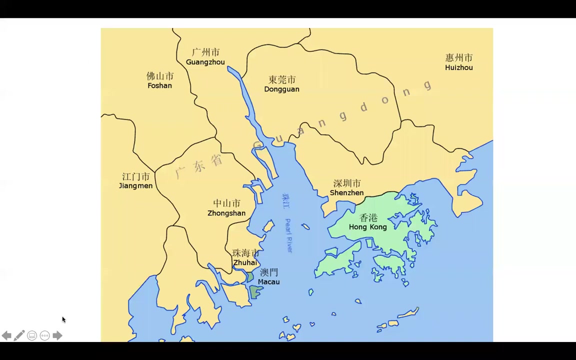 most of our corals are on the eastern side. Anybody want to guess why we only have corals on the eastern side side and not the western side? Neutrin, rich water, currents- okay. Nuclear plant plant okay, Ocean. okay. The answer is this. The answer is: I think Sharon is. 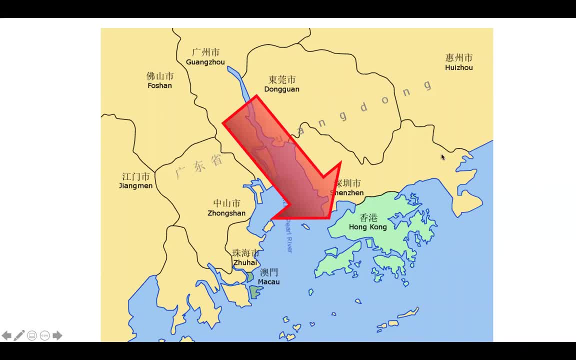 correct? The answer is because we have Neutrin rich current from the left-hand side, from the peripheral Delta, so that means the salinity is lower there. so it's not ideal for coral and it's also very turbid. so that's why most of 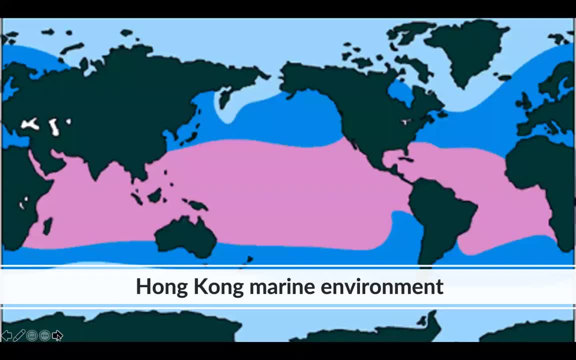 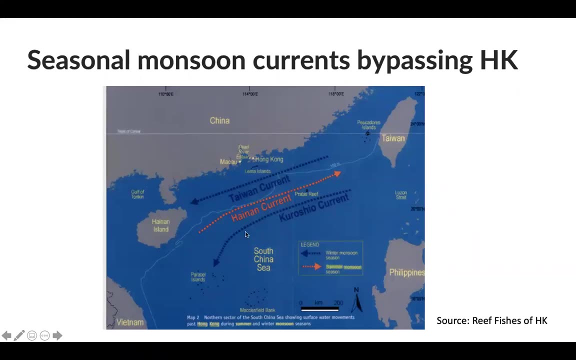 the coral we find is on the white hand side. So Hong Kong is in the subtropical area. We have the influence of both the current from the north. we have the Taiwan and the Coral Shell current, which is a winter monsoon current, and then we have summer current from Hainan. 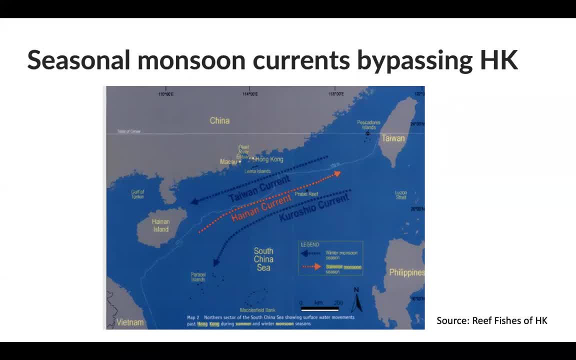 Island. So because of the monsoon current, even though we have a winter, the water is not too cold. so that's why, actually, in the winter in Hong Kong, you find quite many baby fish that are being brought by the Coral Shell and Taiwan current. so that's why, Hong Kong, we have such diversity. 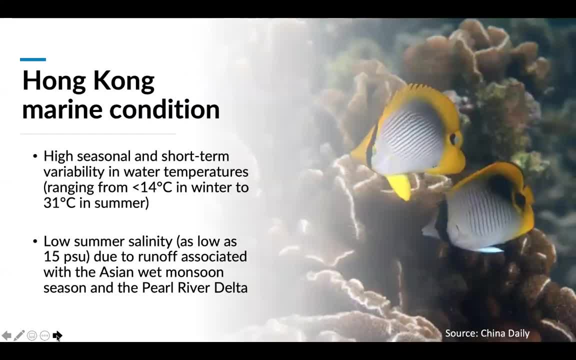 because of the mixing of the monsoon current And if you look at the temperature, our water temperature vary from 14 degrees to 31 degrees uh in the summer, and we also have lower summer salinity due to the runoff from the per river delta. so this is, uh, just a little bit of background before. 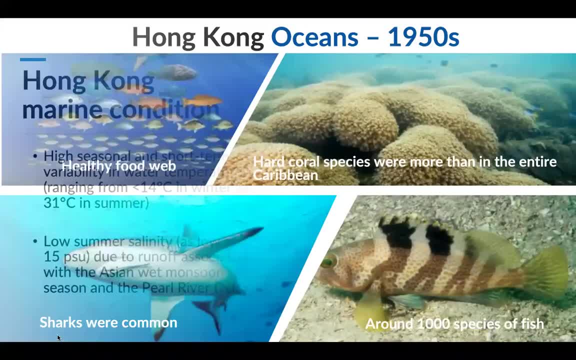 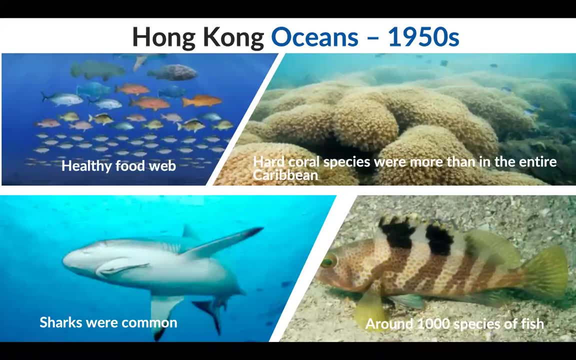 we talk about biodiversity. so in hong kong, uh, we used to have a very healthy food web. uh. uh, we have more uh. sharks were very common uh in the 70s, in the 50s, and what happened is there was over fishing uh, and a lot of over dredging, and our 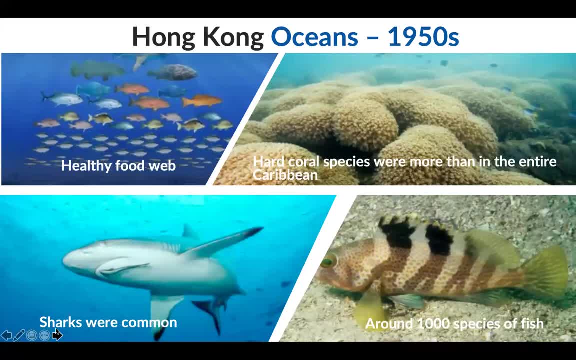 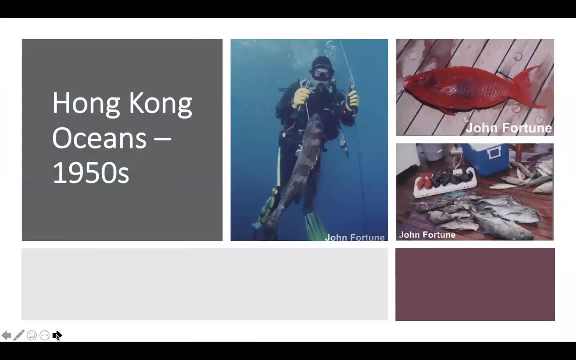 corals are not as soon as as good as as before, but i have to say, because i think of the fishing ban and uh, maybe this year also because of covert, i have seen uh better biodiversity and better visibility just this year. uh, this is a picture from my friend john fortune. he is a very 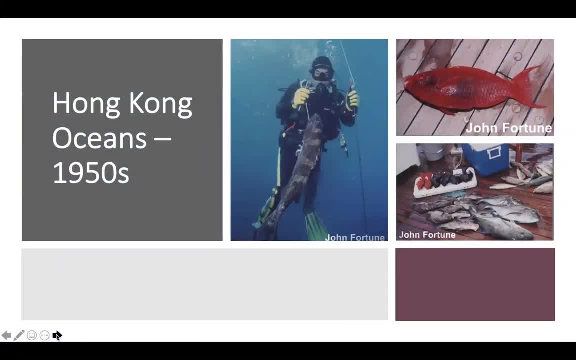 famous diver in hong kong. uh, this is his picture in the 70s, as you can see. uh, the grouper he was, he, he, he was, he was catching- was massive in hong kong. it's very hard to find with fish that are that big now. 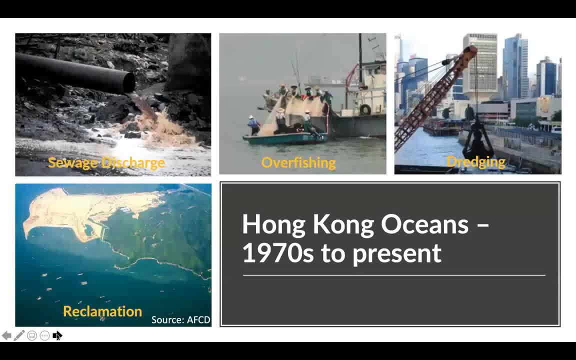 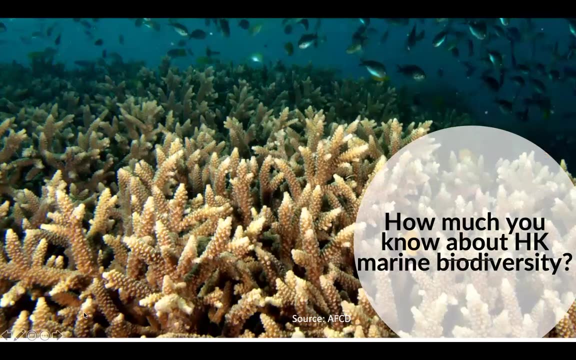 because they are being overfished. and, as i said, uh, these are some of the problems, some of the uh pressures uh that the hong kong uh oceans face. so now, uh, let's go to the meat of the presentation, which is the marine biodiversity. so, uh, i'm not going to be very scientific. 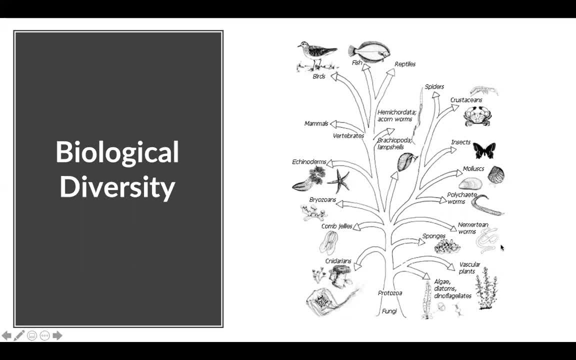 about today because it's going to be an intro class, but i do want to introduce. there's this: uh, we call it phylogenetic tree, so all the animals, uh, from fungi to protozoa, then it becomes cnidarian, then, uh, uh, it, uh, it gets more and more complex. we. 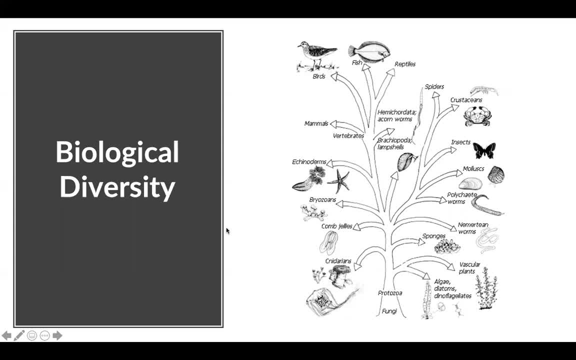 have econoderm. then finally we have fish and mammals and all that. so we're not going to talk in depth, but this is just to give an overview of where these animals come from. so i'm going to start actually with the most sexy stuff for us. oh no, not a sexy stuff, but uh. 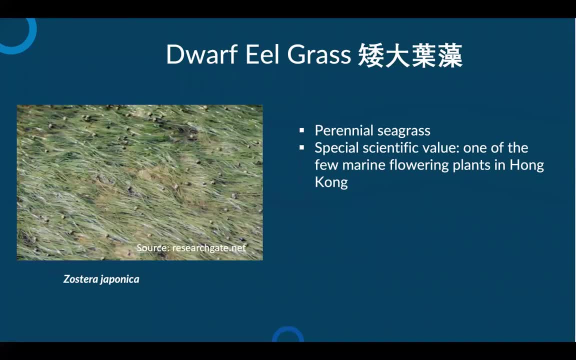 but, but, but then less sexy stuff, uh, so we're going to talk with eelgrass as well. so they don't look very, they don't look very, uh, very important. they just look like a piece of grass, but they are actually very important because they stabilize the coastline and sediment. 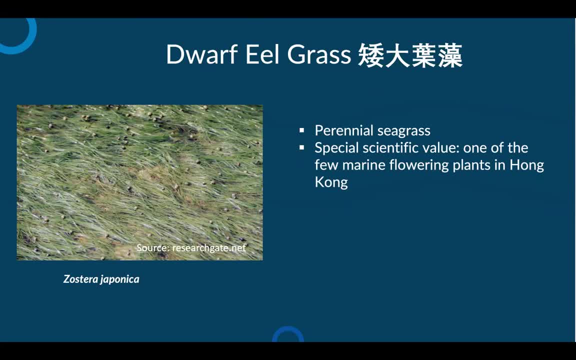 they are also a feeding ground for a lot of small fishes. this dwarf eelgrass is the only type of seagrass in hong kong that are able to pollinate underwater, so you do see them quite a bit. this is brown seaweed. they are not seagrass. uh, they are called ma mei chou. 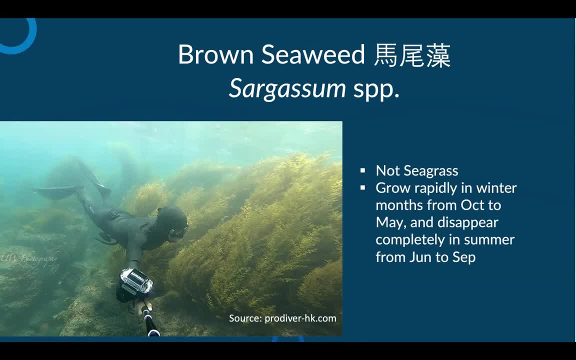 in chinese and they are very pretty. they go rapidly in the winter months. this is a one of my friend who is diving uh in in this, uh, very nice sarcasm bed. uh, they are not actually, uh, uh, uh, true plant, because they don't have leaves, stems and roots. uh, they're just very. 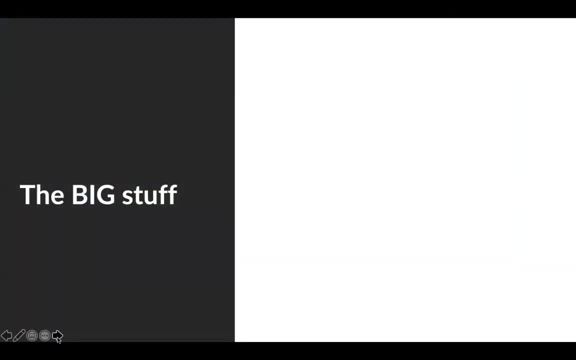 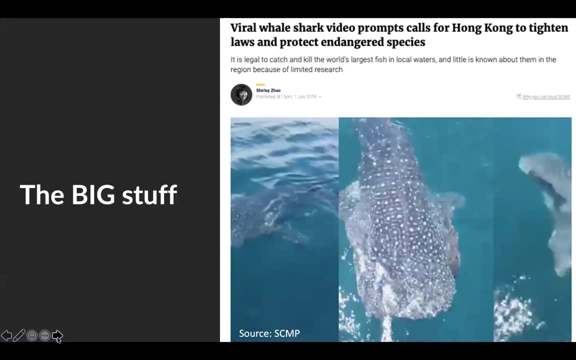 very temporary, okay. and now the big stuff. so in hong kong we have sightings of, uh uh, whale sharks. so this was two years ago. uh uh, we, and i think just a few months ago, somebody spot that near llama island and as well a whale shark, and we also have tiger shark. so this 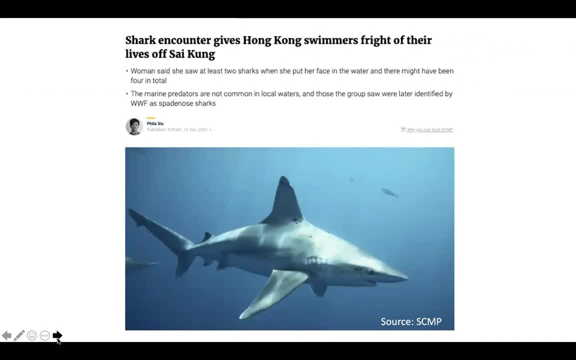 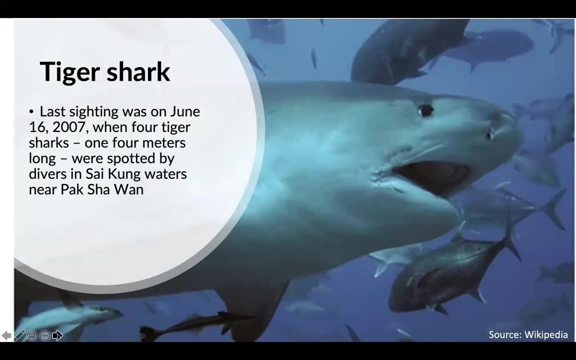 was just uh, two, uh, uh, two months ago in june, that, uh, that, uh, a swimmer was sawing, uh like a tiger shark near her, her, um, uh, her face, and similarly, uh, yes, this was tiger in pakistan one. so we do have very big stuff in hong kong, and if you wonder how many sharks we 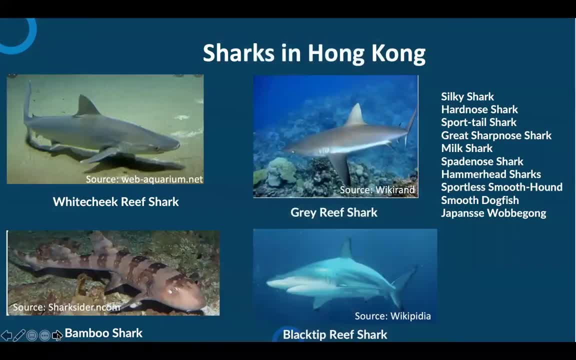 find in hong kong. in total, there you go. these are all the sharks in hong kong and i must say some are more popular, uh, more more common, like the black teeth shark is pretty common, uh, uh, uh, in hong kong shallow waters, you find them in the day. 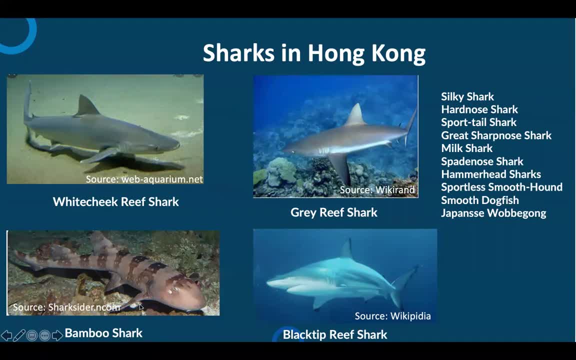 uh, this is bamboo shark. they are common at night. i have seen quite a many of them when i go night dive. uh, so the sharks are not as a decent, uh, a harmless shark. uh, they won't attack people actually, um, uh, so, uh, actually it's not that hard to see them in hong kong. 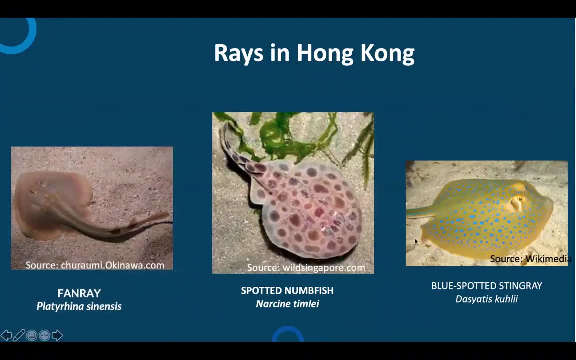 we also have rays in hong kong. uh, these are very pretty rays uh. this one, uh, blue spotter stingray is very common in the shallow water, uh, and they are just very pretty to watch and they're like some. some of them are expect, expect as big. 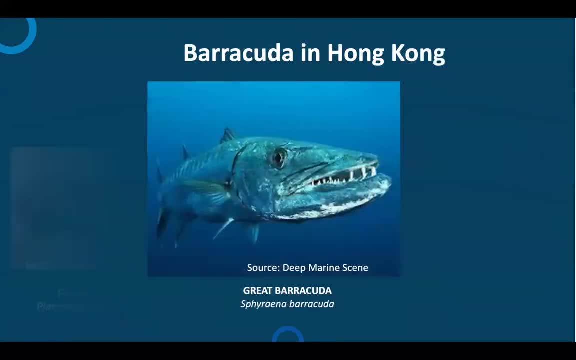 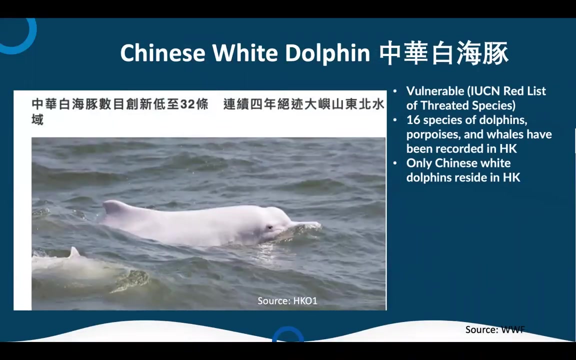 as a table. we also have big stuff like barracuda- uh, they come in a school of them. uh, not exactly very common, but they do live in hong kong waters and some people do fish them- and chinese white dolphin- i think a lot of people in hong kong are. 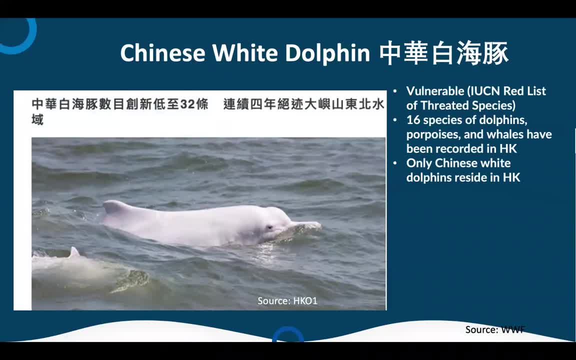 heard of them, uh, and and, and i don't know if you know why they are pink and the reason is because they're actually white, uh, uh. but when they come to the surface, because, uh, the skin is very thin, uh, so the blood dilates, so they look pink. uh, they are very uh, they are just 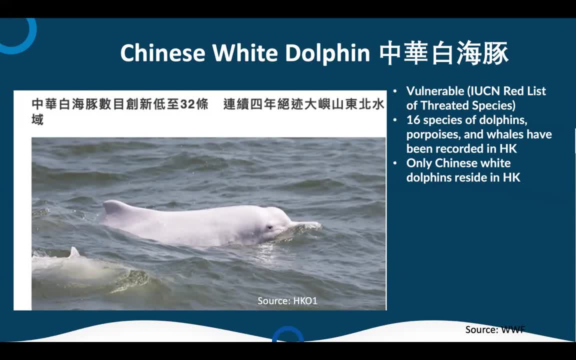 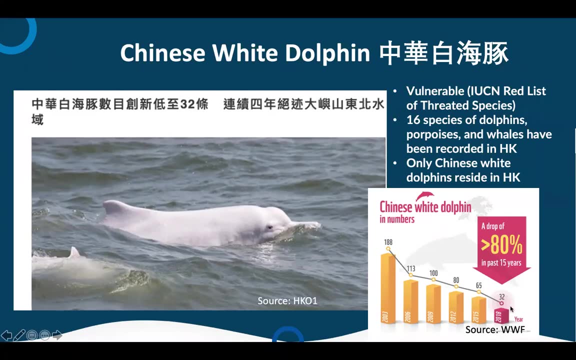 actually uh discovered, just like 20 years ago when they built the uh uh uh new airport, but now they have become uh very endangered. so from 188 species- uh numbers- we have a lot of yellow turtles where we first discovered them. it has dropped to 32 and i think the number is even lower this year. 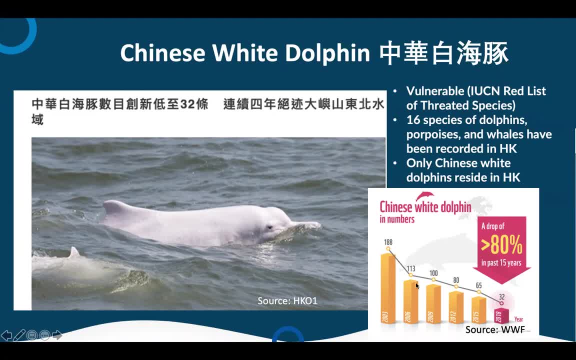 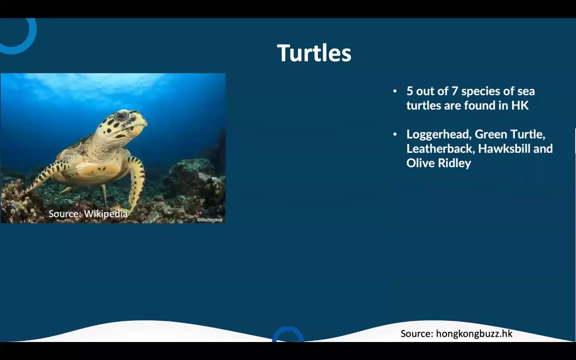 uh, this year there has been several news that there are dead dolphins found in the beach. so, uh, because of all the reclamation, uh, all the building in the in the western part of hong kong is really not helpful for this chinese white dolphin. we also have turtles in hong kong, so, uh, we have loggerhead leatherback. 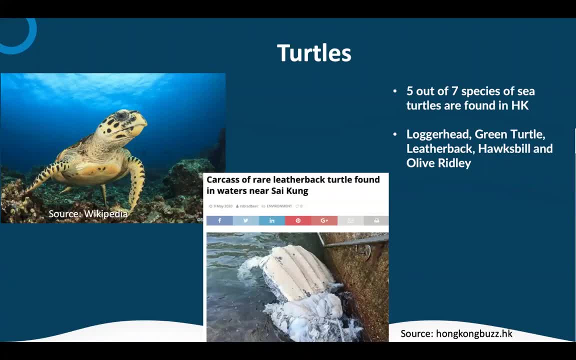 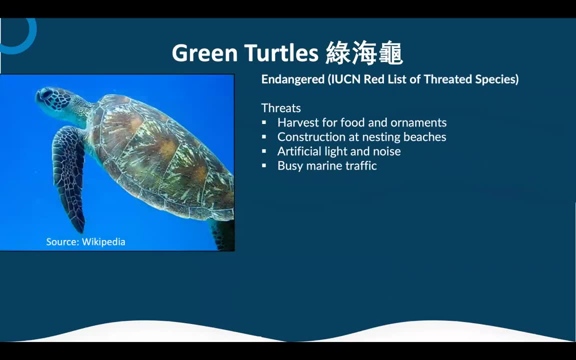 and this was just in may this year- there was a a rare leatherback turtle fine near the beach cycle. So we do have quite a bit of turtles in Hong Kong and the most common one is green turtle. They are also endangered. A lot of them got trapped by. 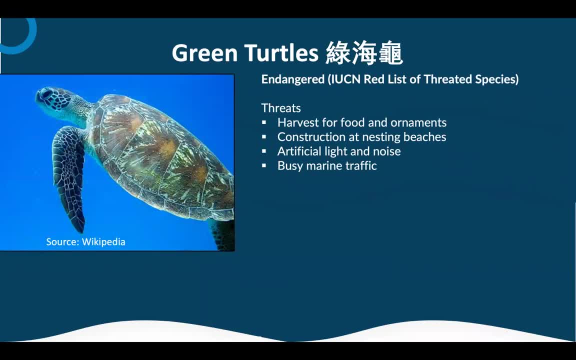 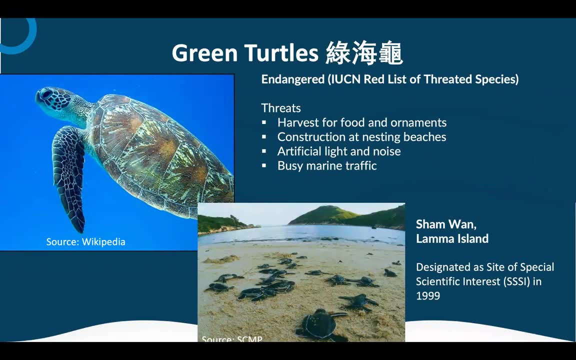 plastic as well In Hong Kong. we are the remaining few sites in southern China sea where they breed and then also not nesting every year. So we are really worried about the population. but if you are really interested to see them, maybe at a certain month you can go and find them in the someone. But just remember. 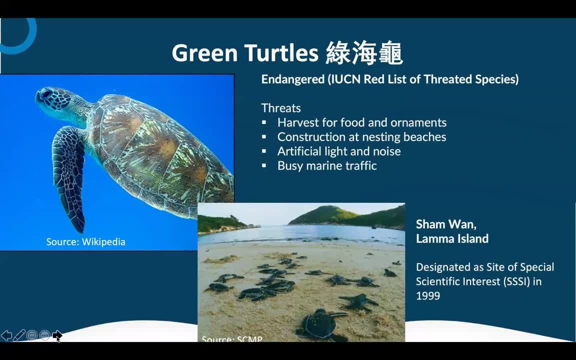 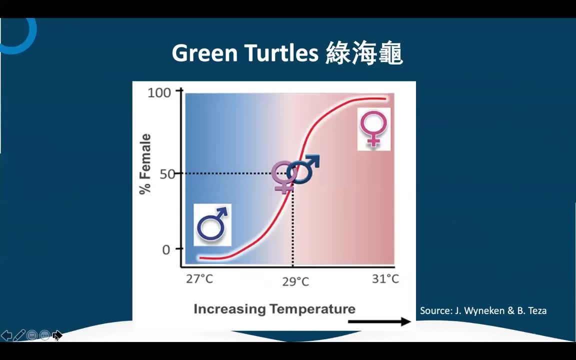 them, try not to disturb their habitat too much. This is another diagram I want to show you. This is a temperature dependent sex graph. So the green turtle at the lower temperature, all of them are male, and above a certain temperature, all of them are female, And the point of this is because of climate change and 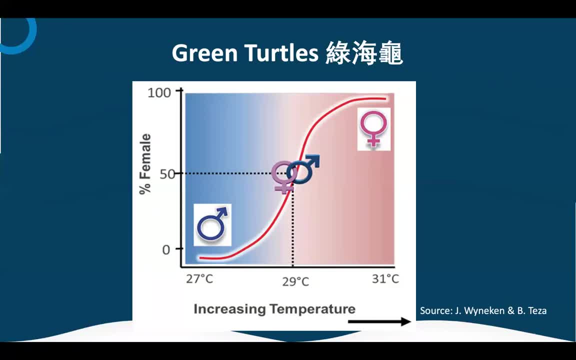 which, no, Hong Kong just had the hottest July on record- then it means more and more turtles will be female And that's not a good thing, because if you have only females and not enough males, that means the sex ratio is not an ideal ratio for them to mate. That means less and less green. 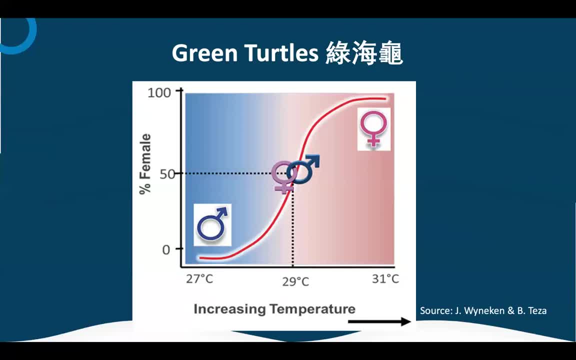 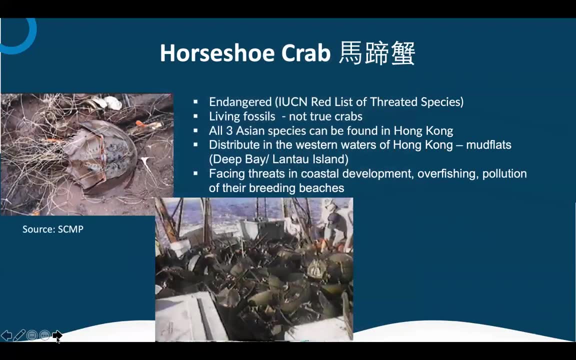 turtle. So, yes, climate change is affecting Hong Kong biodiversity quite a bit. And now we have horseshoe crab. Horseshoe crab is one of my favorite species. They are called crabs, but they're actually not crabs. They are actually. 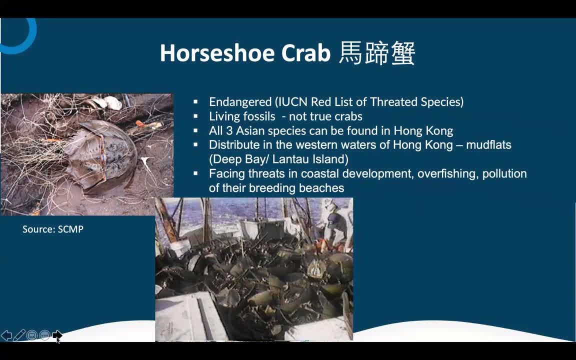 relative of spider and scorpion. They are actually more than 300 million years. They're as old as the dinosaurs. They have disappeared since the 1980s but have recently been found in some areas. However, there's a lot of threats about. 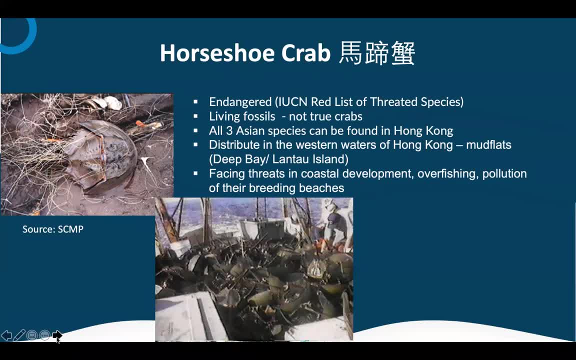 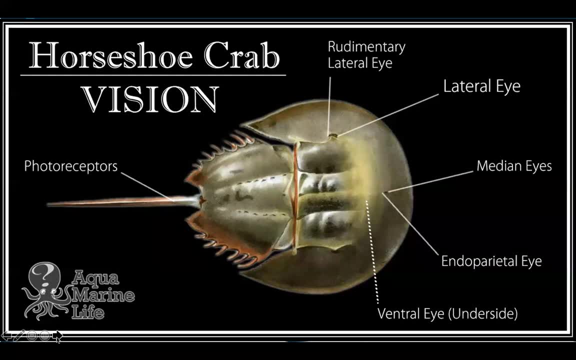 their habitat and in the later part of the presentation I will show you where they're really being disturbed. So horseshoe crab- just one front-footed crab. fact, they have a lot of uh, they have 10 eyes. they have 10 eyes in there. they have very good vision. 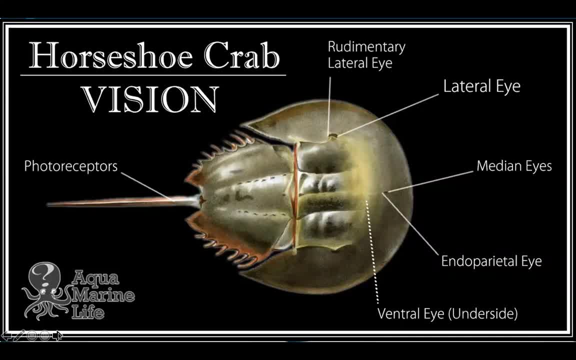 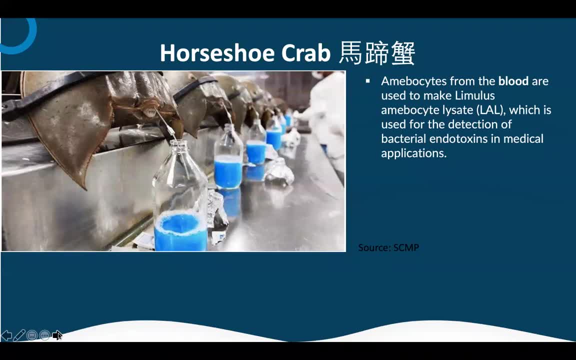 uh, so, and and they are very smart animals, so it's unfortunately people, uh, they, we call them milking. they were milking them for the uh, for, for for their blood, and their blood is blue in color because, uh, not like us where we have hemoglobin, where our blood is made of iron, their blood is. 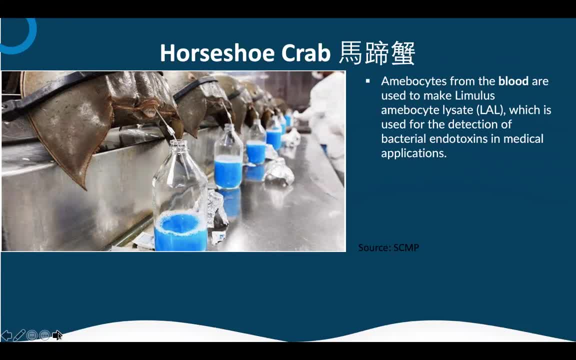 made of cyanide, so cyanide is blue in color and they are supposed to have uh medical value from the blood, which means a lot of people are harvesting them and also the chinese people also cook them as well. so in hong kong in the last 20 years, the horseshoe crab population. 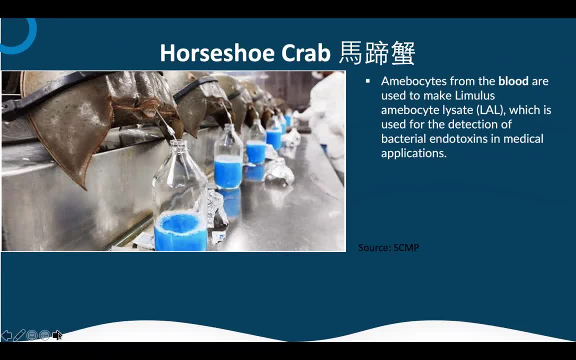 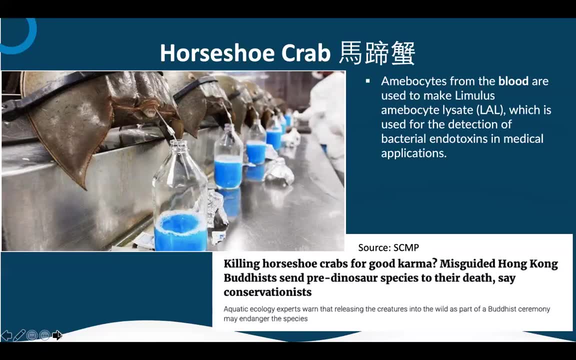 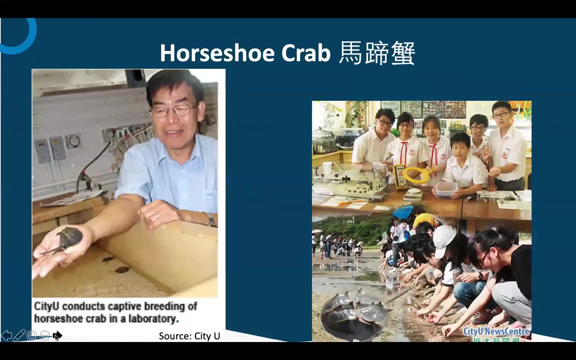 has decreased 90, so this is just to show you how serious uh that they are being threatened. uh, yes, again. uh, some people kill horseshoe crab for good karma. they think that, uh, that will bring them luck, and it's really not a good thing. uh. there is one good news uh that professor uh. 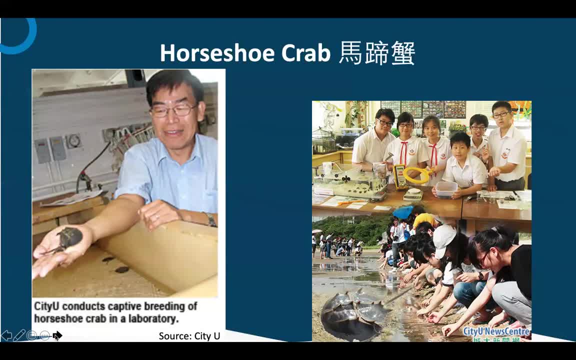 uh yim in ctu, he is, uh, he's a, he's a expert in the horseshoe crab and he uh, breathes this baby horseshoe crab in his lab and until they are- they are a bit older, like a size of his palm, and then 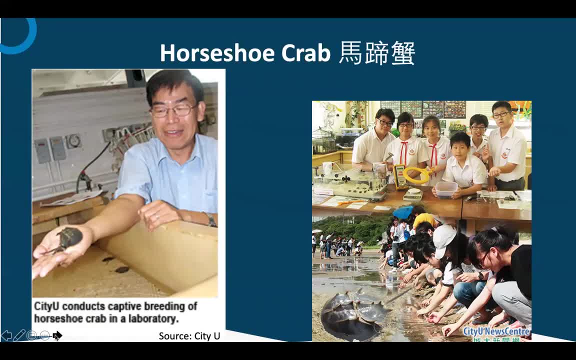 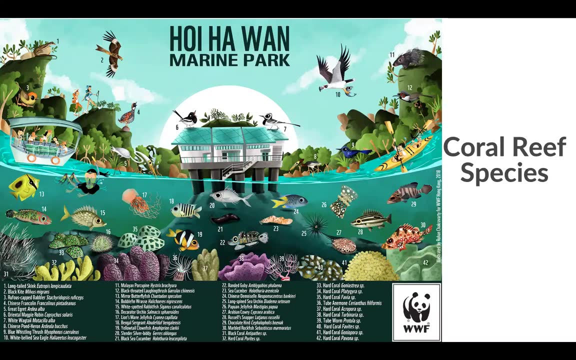 they raise it to the wild, hoping then that will recover their population a little bit. so there are very good people in hong kong trying to to do conservation work to help rescue these animals. uh, now i will talk a little bit about coral reefs. uh, first up is the cec connective. we have a very unique 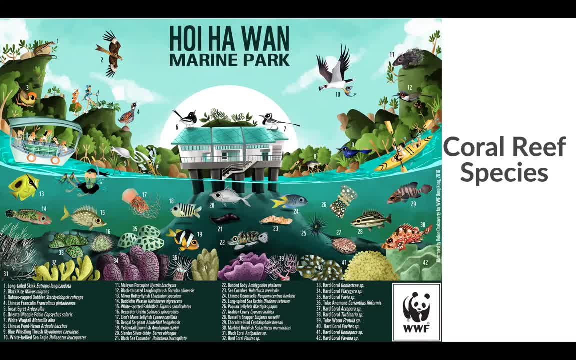 species. uh, this is a diagram from huong hao wan uh. so, as i said, uh huong hao wan is the second most uh 4 paces with the highest biodiversity other than tong peng chou. you can see all these animals just by snorkeling and if you haven't been, i really encourage you to. 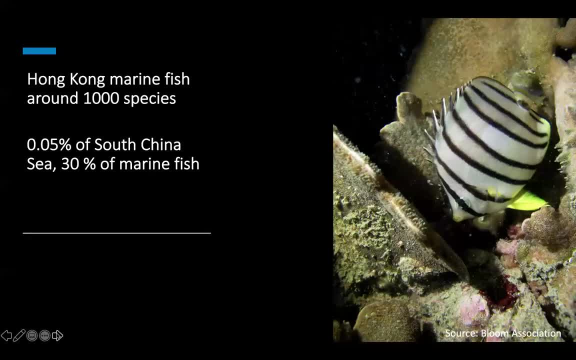 uh, you can also join one of our tours in encompassing, where we go there pretty frequently and will tell you what all these animals are. so, uh, yes, uh, we talked now, we talked about that. hong kong has more than a thousand species of, say, ugh. 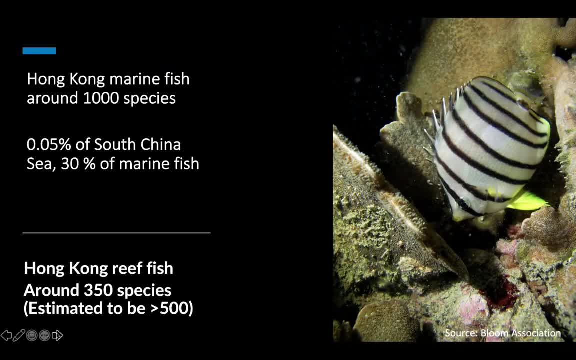 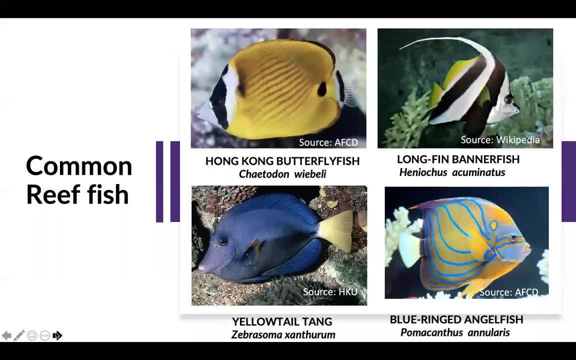 fishes and for with fishes. so not all marine fishes are with fishes, some of them are just oceans fish with fishes. we have around 350 species, so these are some common uh with fishes. you might see them in like finding nemo, finding dory, very like. this is like kind of like a dory. 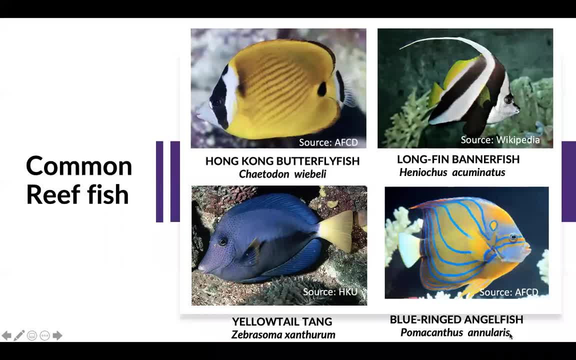 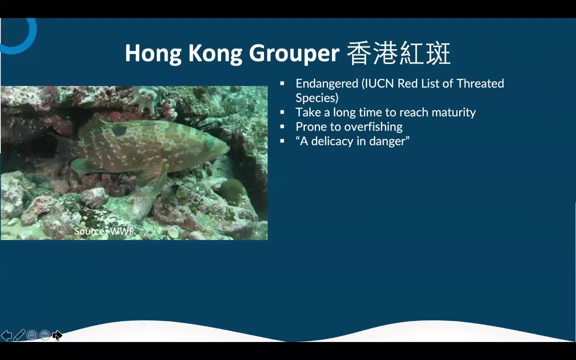 kind of fish. they are quite common and, as i said, uh, their babies are quite common in the winter because of the of of the current. uh, yes, so this beautiful fishes can be seen in snorkeling or diving in hong kong. the grouper, uh, hong kong grouper- is an endangered species. they take a. 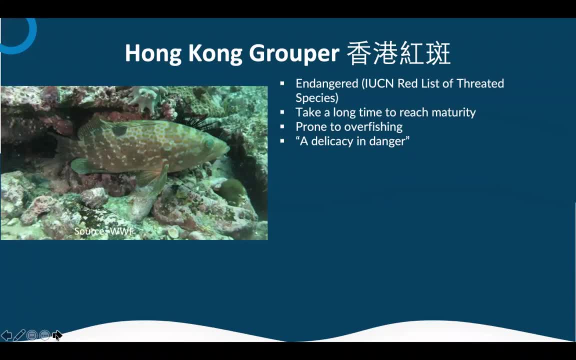 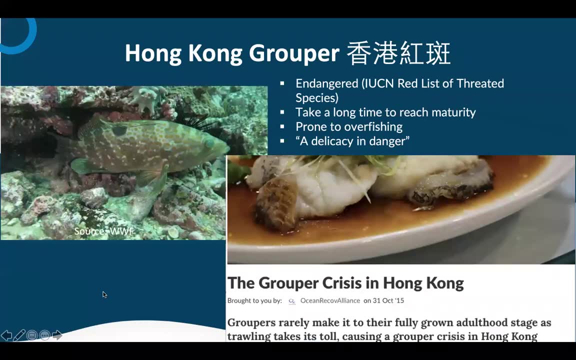 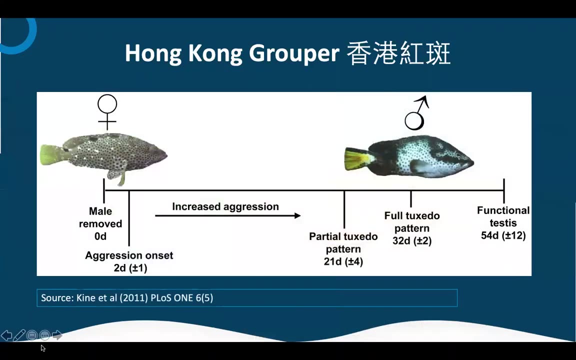 long time to reach maturity. uh, they are also prone to overfishing. uh, yes, uh, so they are. they they're often being caught even before they're making a big size. so again, uh, this is kind of a of like the um total, but this is now, uh, they're determined by the size, the sex ratio. so, uh, when, 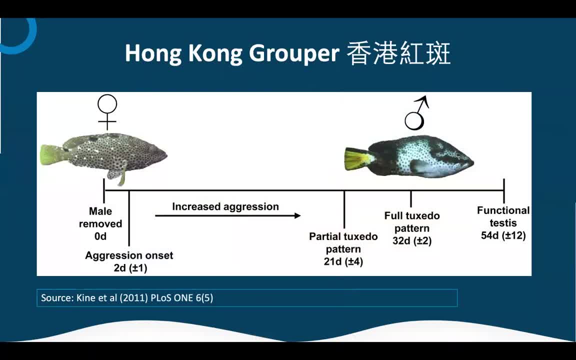 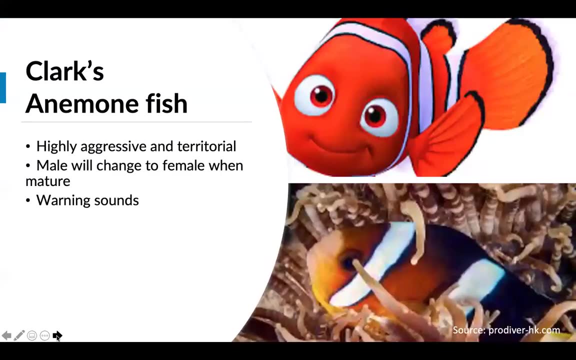 the um grouper. grow bigger, they become a male. when they're smaller, they become female. but the problem is when they're being half uh being fish, or or when they're smaller, then not enough fish become male to mate. so this is another problem of uh overfishing. okay, this is one of my favorite. 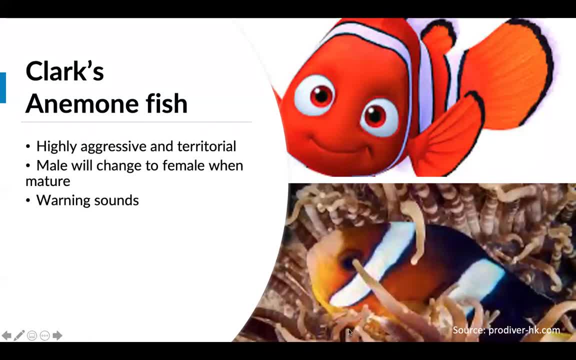 fish. i don't know if any of you have seen it, so question: do you think the this fish on the bottom, which is a common species of uh anemone fish in hong kong, are they the same fish as the dory upstairs? so, yes or no? 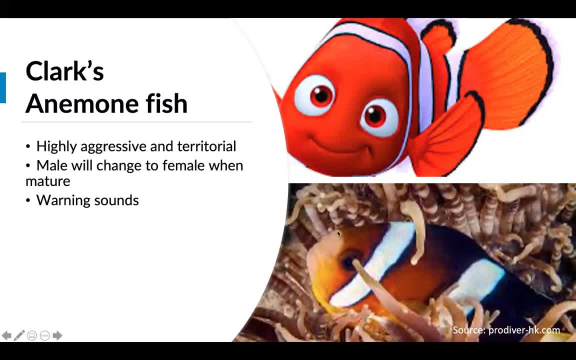 anybody want to guess? is the fish down here the same fish as the fish up here? so it's either yes or no. anybody want to guess? okay, we have some different answers. the answer is yes or no. this fish, anemone fish, is different from the one in the top. this one is called a clarkia anemone fish. 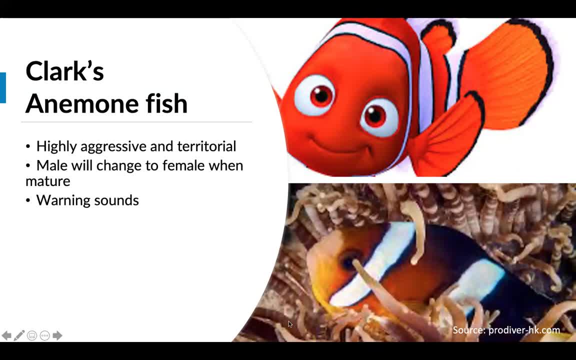 uh, this, this one is the common anemone fish and the difference, this one is all over hong kong. okay, it's like you almost see them in any, every dive. they are very aggressive and territorial, so when you go near them, they will give you like a small bite like this in that, uh, and they also give you. 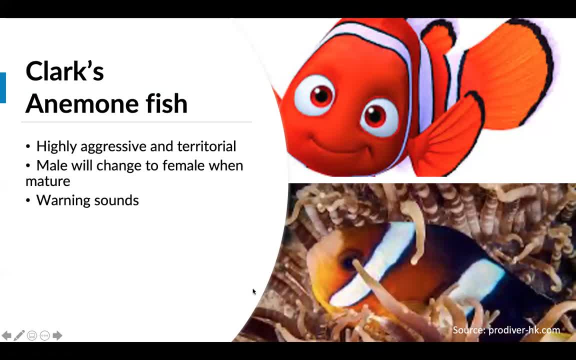 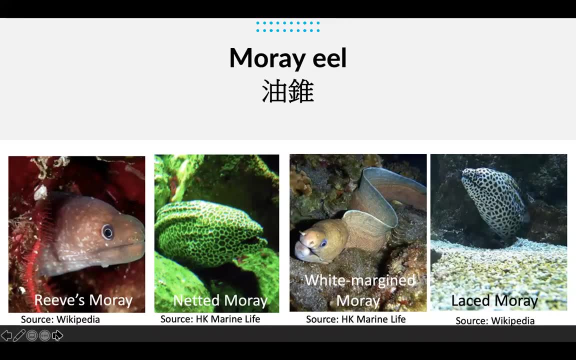 a warning sign when they want to attack you. so, yes, uh, uh, very common. uh, anemone fish in hong kong. uh, these are some ewes in hong kong. uh, they are quite common. uh, they're usually under the rock. uh, they don't attack you if you don't attack them, and they're very beautiful to watch. 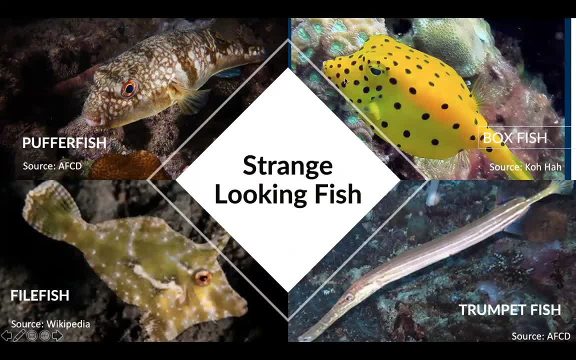 okay, this is some strange looking fish. so i like puffer fish and box fish. they are in the same family. uh, strange looking, uh shape. this is a fire fish which kind of look like a a towel, and then we have trumpet fish. all these are also coming in hong kong, so you might be. 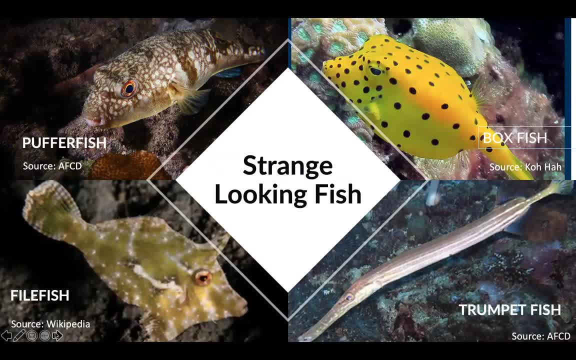 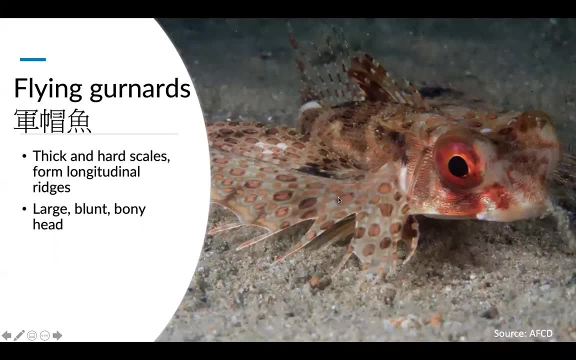 amazed how many things you can see in hong kong. this is a flying gunner- uh, it's called flying because it has this, uh, like a fin that looks like a wing, which likes glide under the ocean. this is very common at night dive. you will see them as well. some people do fish them as well. 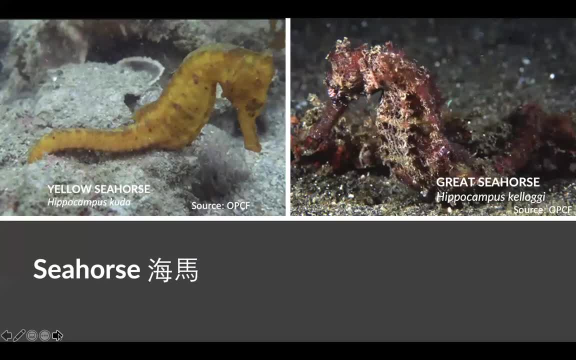 this is seahorse. uh, you might. okay, seahorse is not that common in hong kong. i i would say maybe every 20 dives i see one. but they do exist in hong kong and, just like what you understand with, seahorse is mostly the male which will carry. 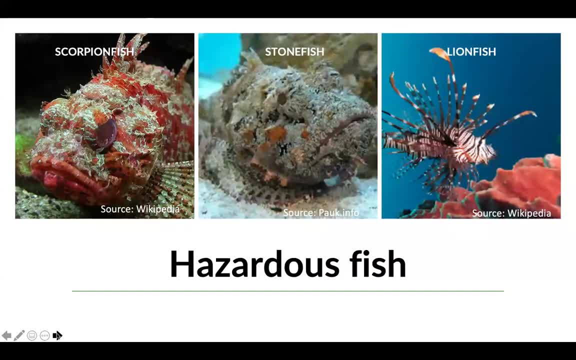 the babies. okay, these are hazardous fish, these are fish you don't want to touch. so we have a scorpion fish, we have stone fish, we have lion fish? uh, yes, and they are poisonous, and the general rule of thumb is: if you don't know what that thing is, don't, don't touch them. they can give you very. 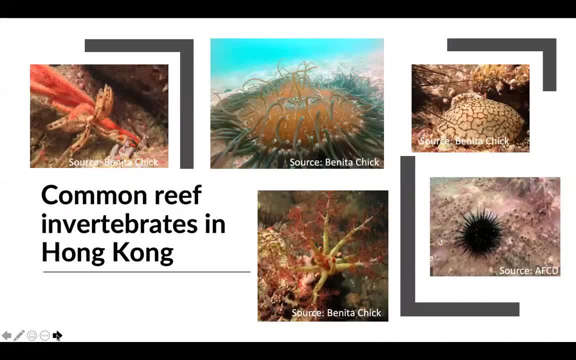 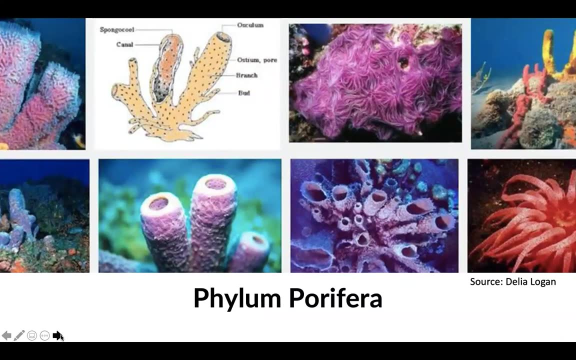 painful, uh feeling. okay. now we're going to talk about invertebrates. so i am an invertebrate person, i'm, i i'm okay with fish, but it's not my favorite. so, uh, we'll start with peripheral, peripheral sponges in hong, uh sponges, so they are very. 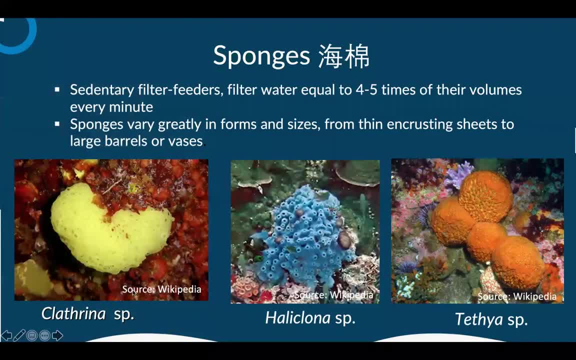 simple in structure. they are filter figures. uh, they can uh uh uh vary in form and sizes. they come in all sorts of colors. so you can see this is all very colorful. uh, sometimes some people miss taking them as coral. but coral actually, if you look closely, usually they pull up like the little. 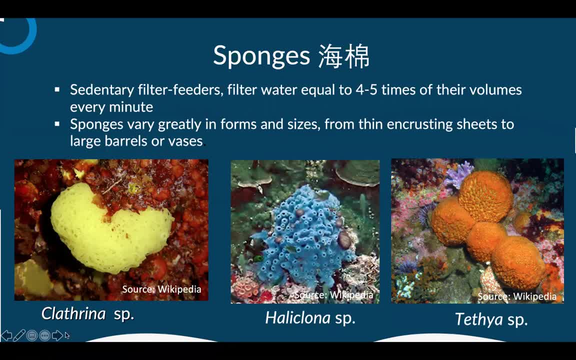 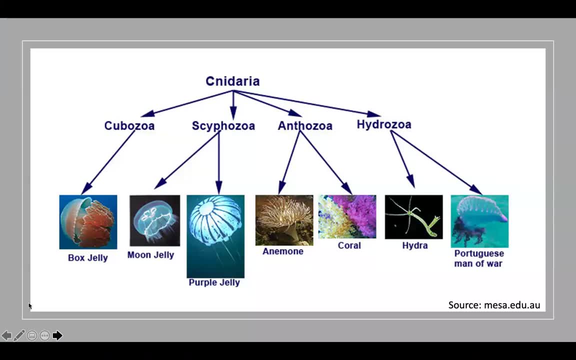 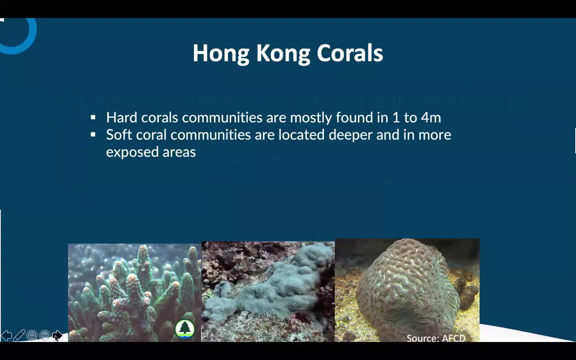 circle thing. it's more regular shape, sponge is more irregular, so that's how you tell them apart. so now we're going to talk about cnidaria. so cnidaria is my favorite phylum, so it have coral, you have jellyfish and all that. so, uh, in hong kong, uh, we have hard corals. uh, they're usually in shallow water. 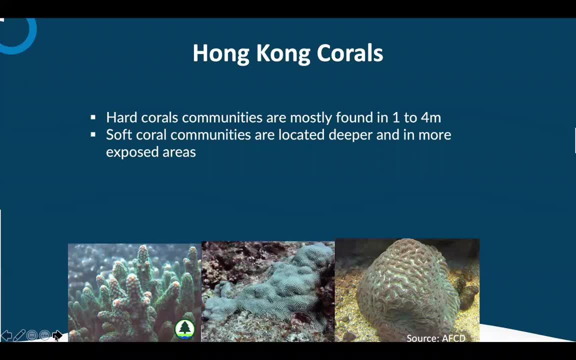 so, in hong kong, when we go diving, uh, it's usually no more than eight meters, because beyond that you really don't see much things. uh, there are more soft coral communities in deep water and more exposed areas. so, uh, corals in hong kong, uh, in other parts of the world you see a lot. 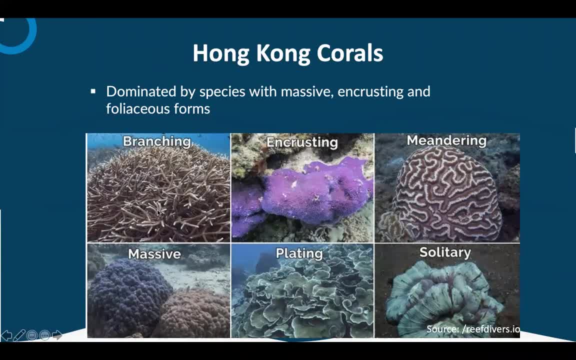 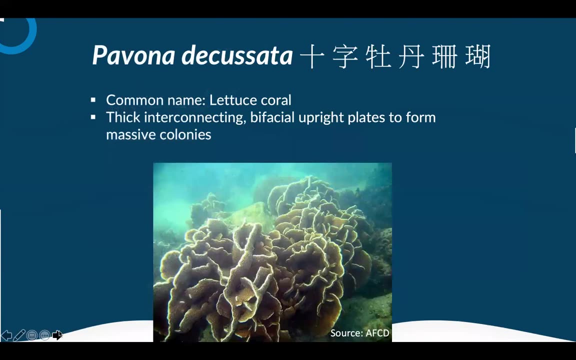 more branching corals because there's more wave. in hong kong we didn't have that much a wave, so most of the coral we see are either massive and crusting or meandering. so this is uh, uh uh. one of the uh common corals in hong kong is called lettuce coral and you can 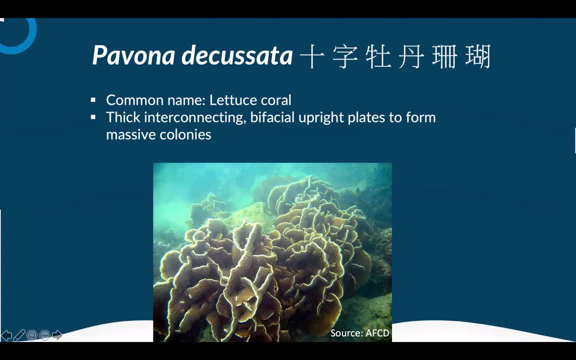 see, the shape is like a lettuce. there's a lot of spaces, uh, in this group of corals that are in the Coral where the fish can take a rest, and very common when you go snorkeling in Hoi Ha or Tong Ping Chau. 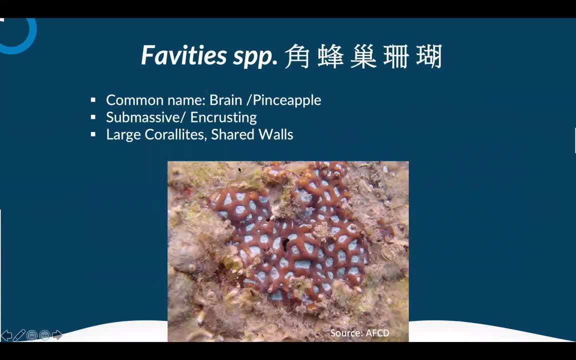 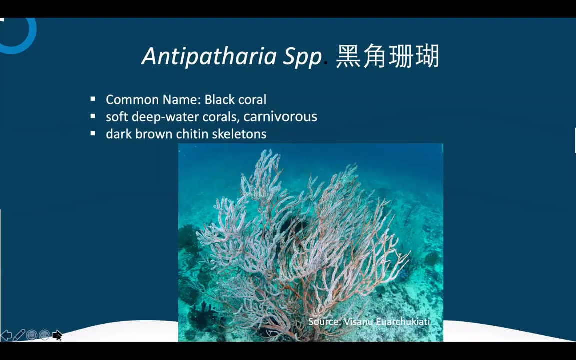 Another coral called phephartis. sometimes it's called a brain or pineapple coral. They are submissive, large corallide shear walls sometimes- yeah, also very common. This is black coral, You might ask. it doesn't look black. 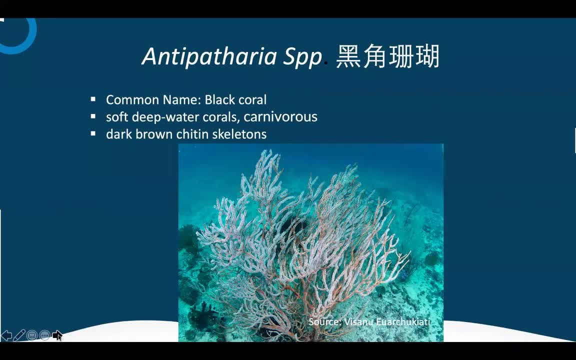 It looks kind of white right. So the reason is because black coral is only the skeleton part is black. Actually, their polyps are white. that's why they look white outside. They're coniferous, so different from the phephartis. 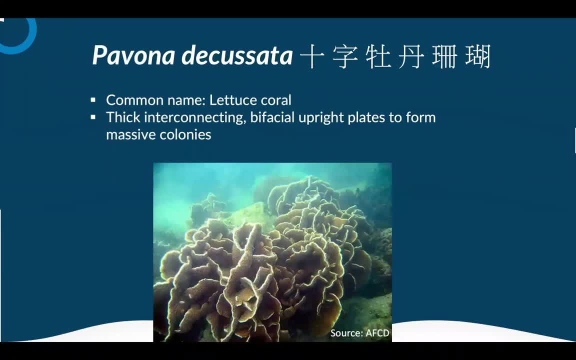 or the profanon coral, Most of the hard coral in Hong Kong. they are symbiotic with algae, So the color of the brown color this coral come from is from the symbiotic algae which photosynthesize, So the coral depending on that photosynthesis for food. 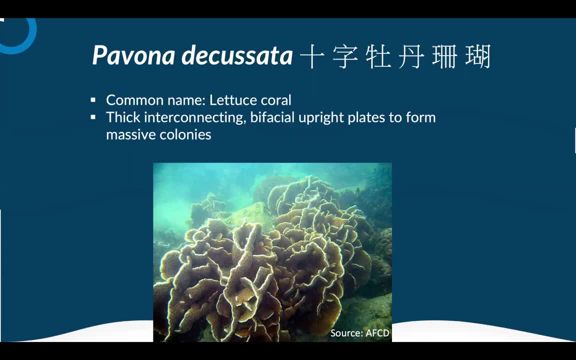 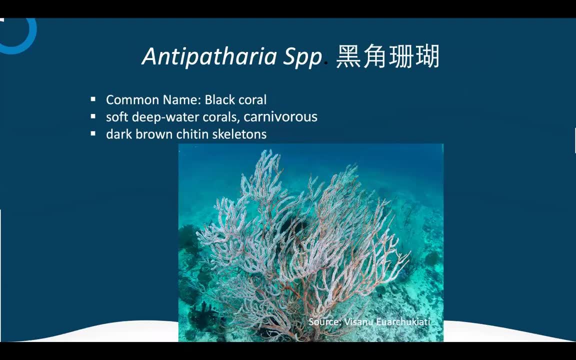 and they do also fit at night, but it's not entirely coniferous, Whereas the black coral, which they are in the deeper water because they don't have as much sunshine, they are almost all coniferous. Okay, and then we have sea anemone. 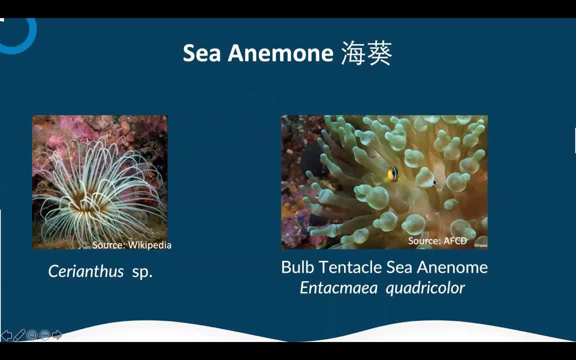 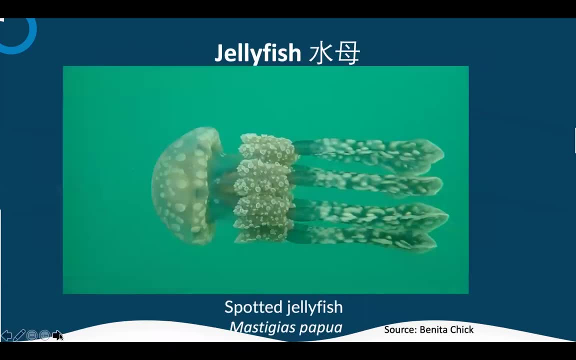 These are the two common type, And this type is very common and they are the home of this kakia anemone fish, which I talked about just now. We have jellyfish and I just want to show you this really cool video. 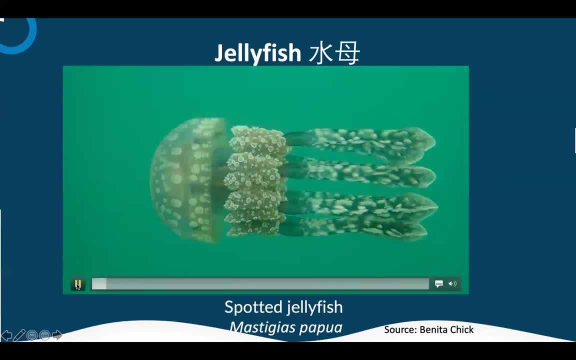 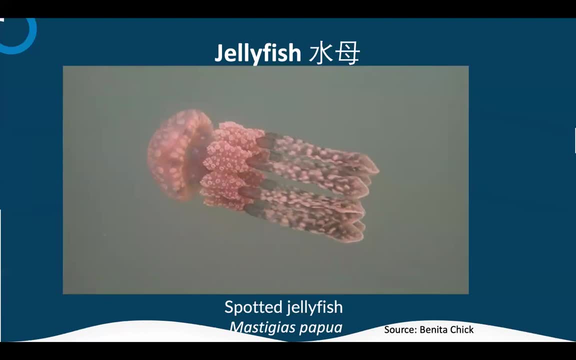 which I took just two weeks ago when I'm in Hong Kong, which I took just two weeks ago when I'm in Hong Kong and you can hear theưa. So again, this is a very common in Hong Kong and I hope you get to see one of them. 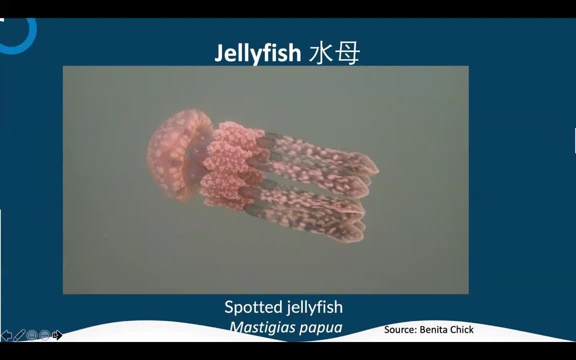 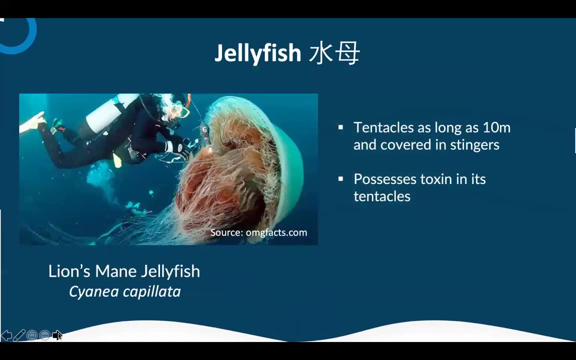 if you go snorkeling in Hong Kong. Oops, sorry. Okay, we do have very large jellyfish. So this is a lion's mane jellyfish. It's as big you can see. it's as big as a human. It's as big you can see, it's as big as a human. 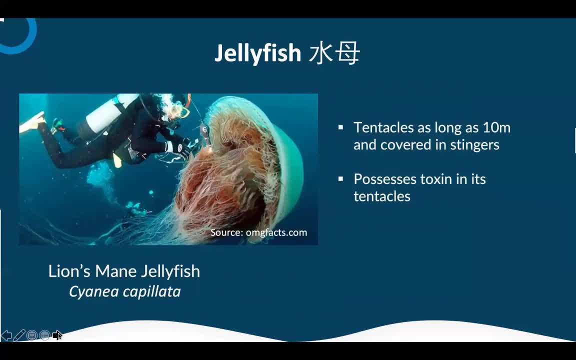 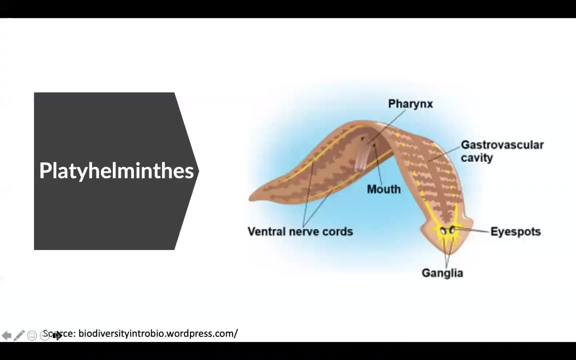 they are highly toxic. so, yeah, this person is not very smart to swim so near them. but I wouldn't say they are very common in Hong Kong. so the other common. the other video: I show you that spotted jellyfish is much more common. okay, and then this is a difficult word to pronounce, it's called platyhelmus. 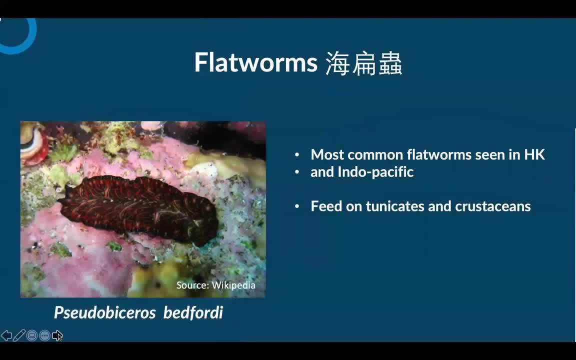 it's a flat worm. so flat worm looks like this: it's flat and it's very pretty. they are very common to see around Hong Kong, Indo-Pacific. they feed on tourniquets and crustacean, and they sometimes swim as well. okay, and then we have annelids. 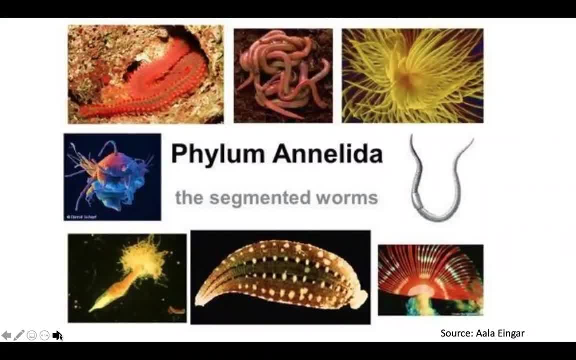 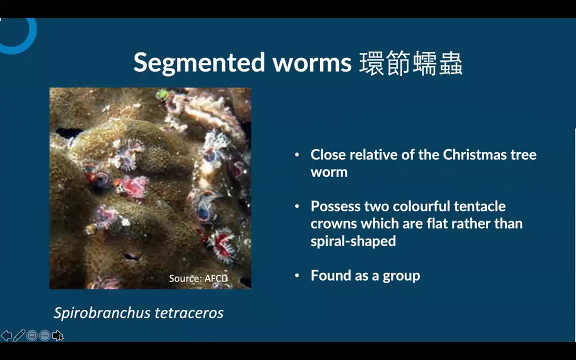 annelids are segmented worm. they are rounded, so not like flatworm. flatworm is flat. annelids are more rounded and they have segments. so for example, this is called a spiral: bronchus tetraceros. it's a. it's a. it's a. it's also called coco. 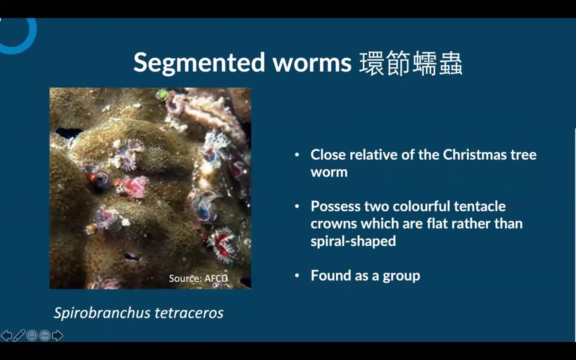 worm. they are close relative of the Christmas tree worm. they have two very colorful tentacles and they're often fine as a group, so they don't worm. I know they look like kind of like jellyfish or I don't know, upside down, but they are worms. so, though the body is buried deep inside this coral, this is the coco worm. 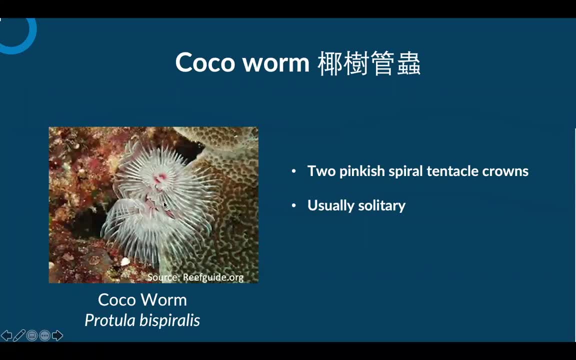 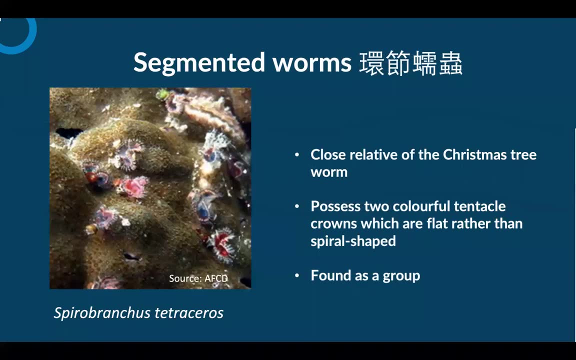 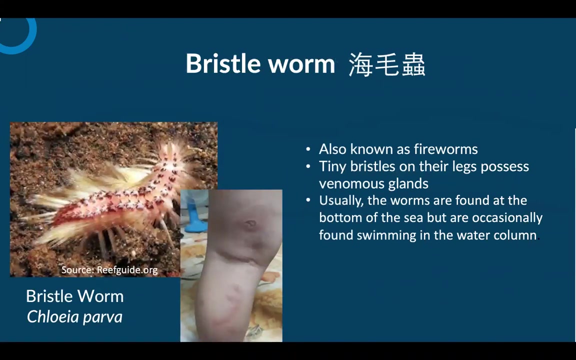 there's a two pinkish, a spiral tentacle crown and this is sort of solitary. so I it's different from this one, this one, the very colorful one. they're usually fine as a group, but this one is solitary. okay, uh, okay, this is bristol worm. uh, this is very, uh, very uh. 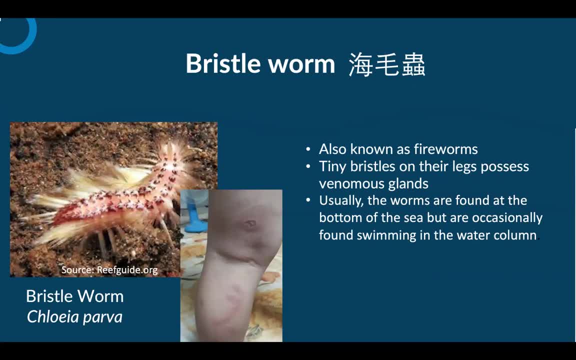 uh uh uh dangerous. they're also known as fireworm, so do not touch them. if you touch them, you end up like this guy: have a really bad scars. uh, they're usually found in the uh bottom of the sea, but occasionally they're fine swimming in the water bottle. so all these 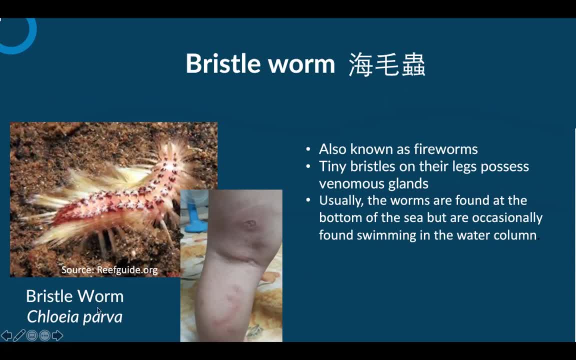 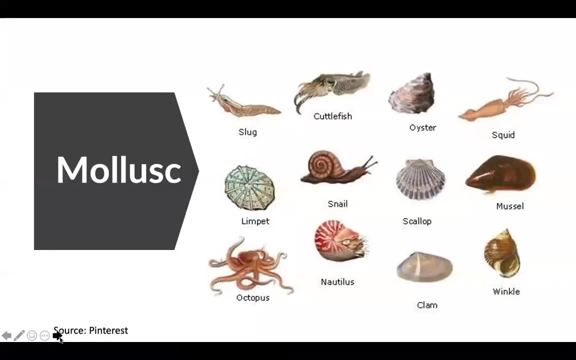 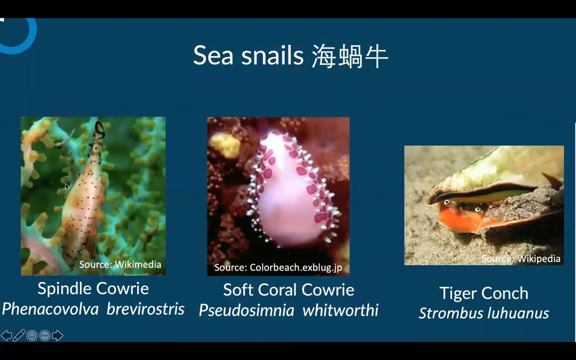 crystals. if you got biting them, i think is as painful as the lionfish. okay, morris. uh, there's a lot of things you can eat here. i think some of you can recognize this. so, uh, we'll start with sea snail. so we have something called a cowie. they are very nice, uh. 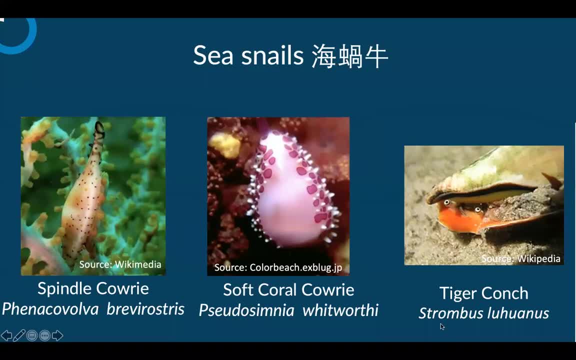 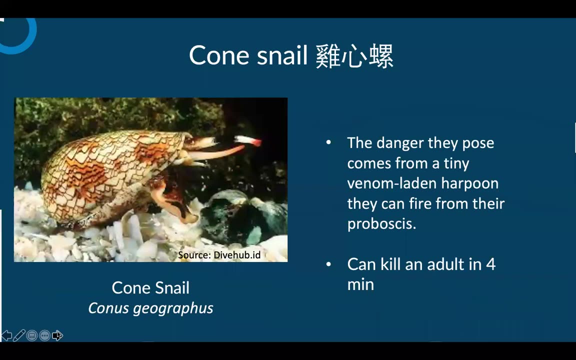 fin shape, and this is a soft coral curry, again very colorful. and then we have tiger crunch, which is kind of like having this Small eyes near, the near, near its shell. This is coals. now you don't want to mess with this. they are also very dangerous. they can kill an adult in four minutes. 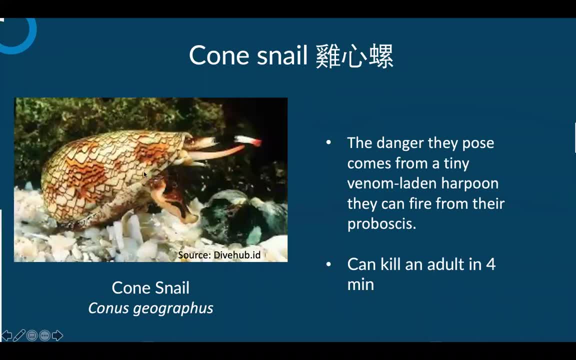 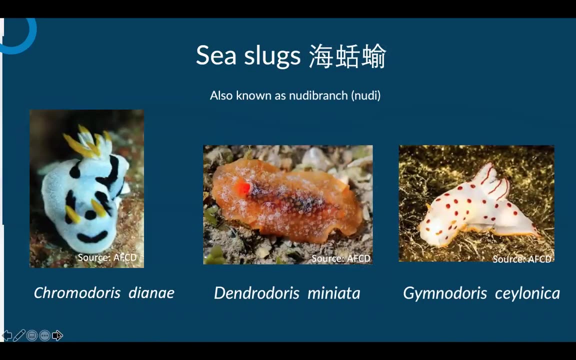 So if you recognize some shell like this, do not go near them. They don't. they don't want to attack you, they want to attack fish, but if you harass them they might. so yeah, Just some hazardous animal you want to be aware of. This is sea slugs, one of my favorite as well. I think they're very photogenic. 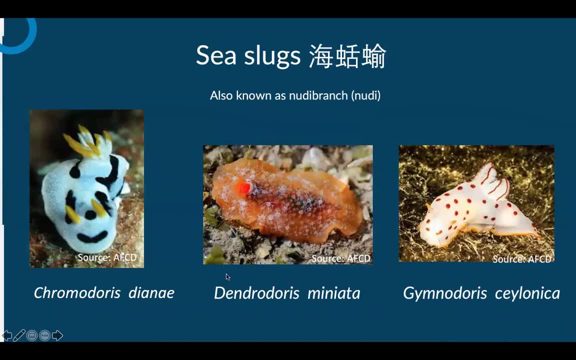 They are like like kind of a snail without the shell. So they come in all sorts of shapes and color and you can see like this, two antennae and like a little thing here. Yes, Not exactly the easiest to find, they're usually just like like, like the size of a fingertip. 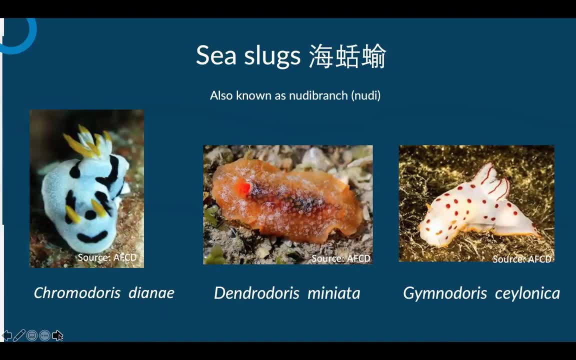 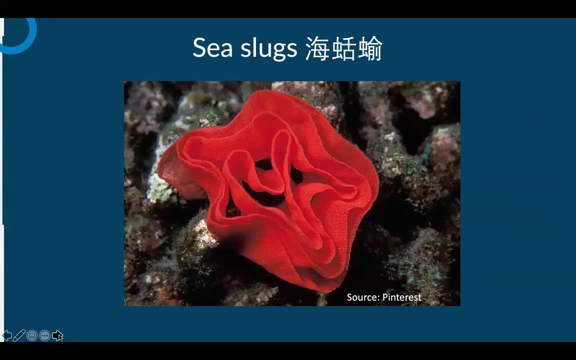 So you need to have very good eyes to find this. But if you cannot find this, you can find a relative. Oh, One more, one more side. This is an egg mass of a sea slug. So it doesn't. If you see that in the ocean, you might not recognize what it is, but it is an egg mass. 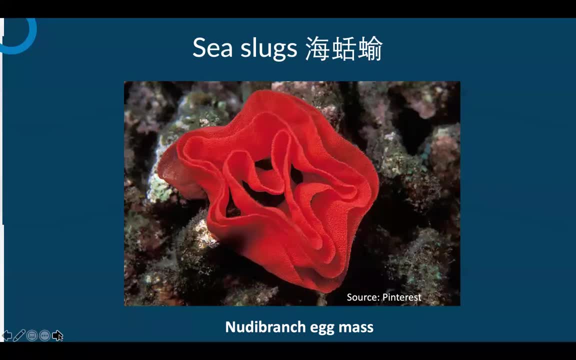 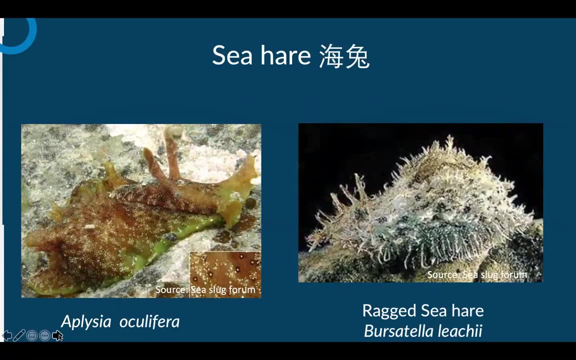 Yeah, Okay. Yeah, this is a nudibranch egg mass, okay, and if Nudibranch is too small to see, you can see sea hare. They are much bigger. They are the size of your hand. They are less colorful. They're usually greenish or brownish in color. in Chinese We call them hoi tou, like a sea rabbit. 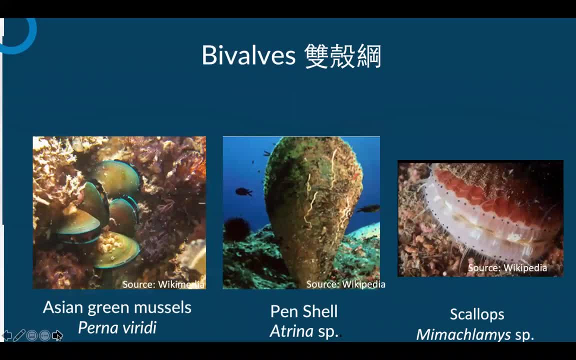 Yeah, Yeah, Okay. and then here are some things you can eat. This is Asian green mussel. quite a bit of a. ladies They usually take this and they go home and eat. this is a pan shell. So when Chinese, because out top so they're like a pan that I stick in the ocean again. 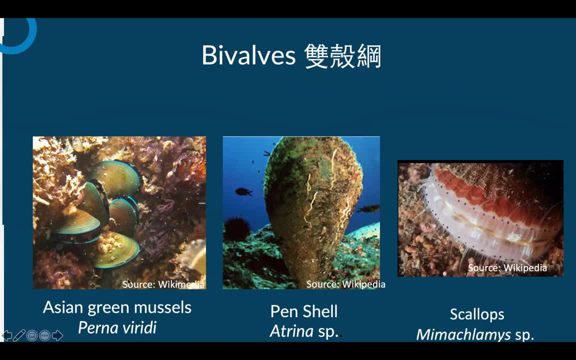 They're quite tasty, but they are more endangered. and this green muscle. So if you are going to eat something, I would recommend green mussel and our pan shell, because pan shell they are much harder to grow, so I would recommend green mussel. And then we also have some scallops as well in Hong Kong. 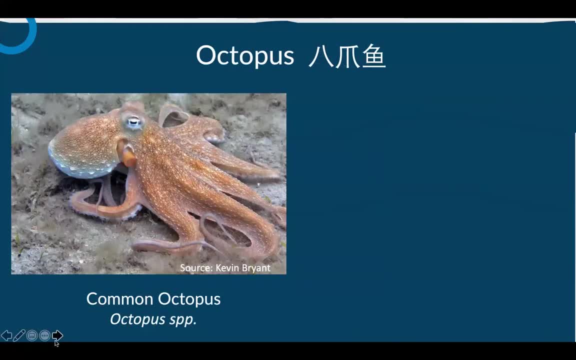 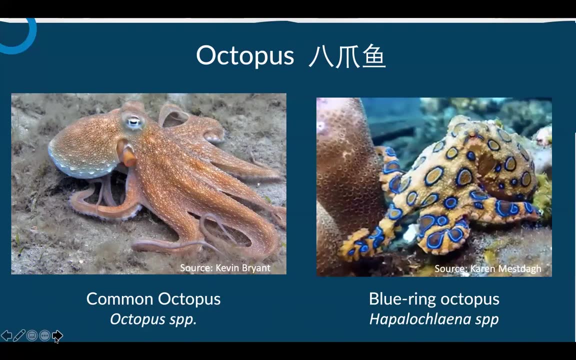 Octopus. Octopus is common in Hong Kong. Some of the octopus you see on the market may be from the Hong Kong ocean, But you do not want to touch this octopus. The blue-ring octopus is extremely dangerous and poisonous as well. 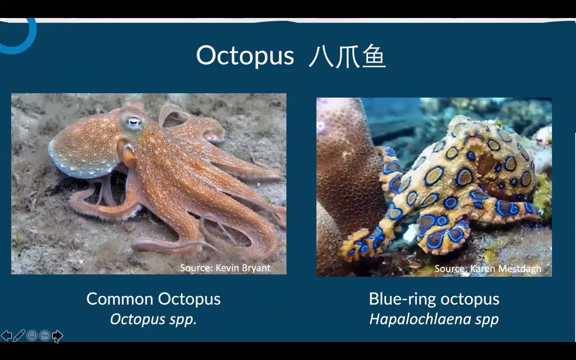 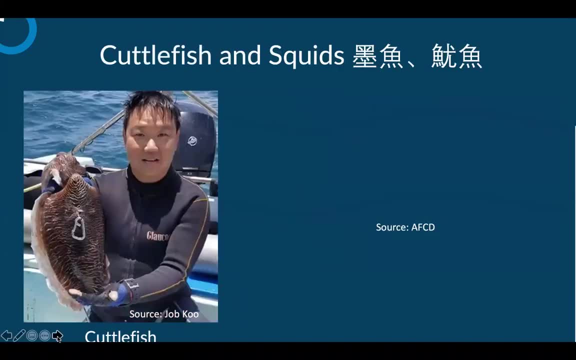 It's not very common, but they do exist, So if you see any octopus with blue-ring, please stay away from it. This is a cuttlefish. This is my friend, Job Koo, on the left. He is holding a very big cuttlefish And the difference between cuttlefish and squid is cuttlefish have a cuttlebone, so they are much. 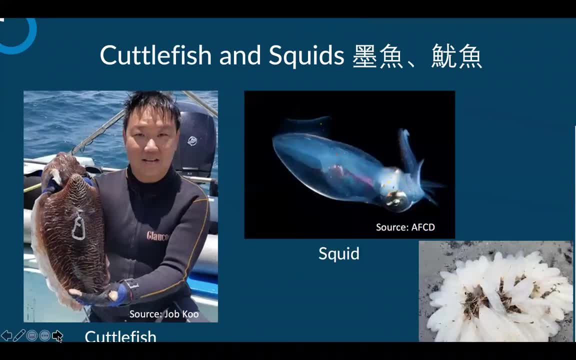 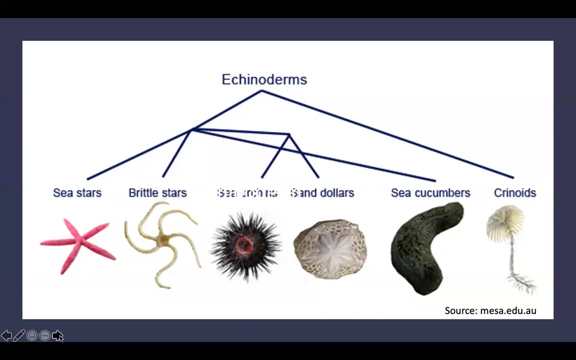 thicker and heavier. And then we have squid, And if you see this on the bottom, this is a squid egg in the bottom of the ocean, so they look like white bubbles, Okay. and then echinoderm. Echinoderm are things with. 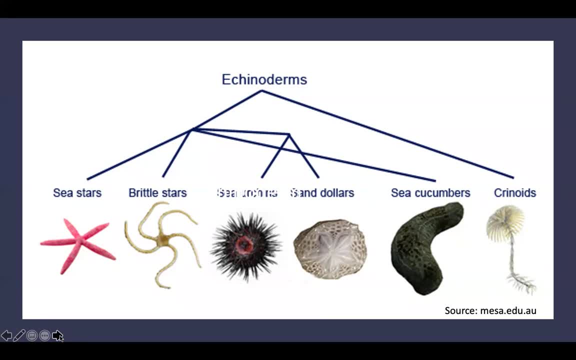 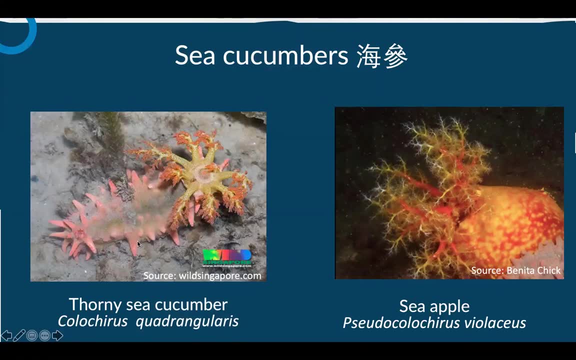 with hard exoskeleton. So this one is common. I mean, I know a lot of people think of sea cucumber as like black, really boring things, but they actually come in all sorts of color And I'm personally quite passionate about sea cucumber. 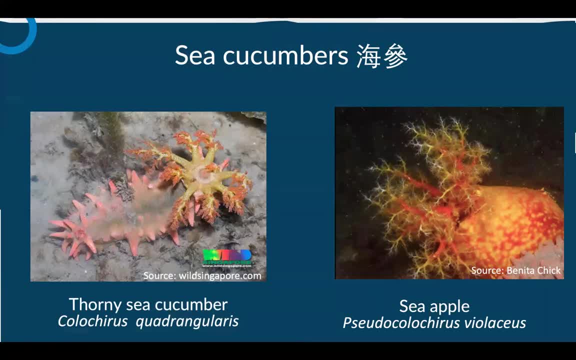 My master is on the genetics of sea cucumber in Indonesia. I think they're fascinating. So this one on the right, the sea apple, is a picture I took in Hong Kong. So these tentacles they do the feeding. But if you mess with sea cucumber, they will mess with you as well. 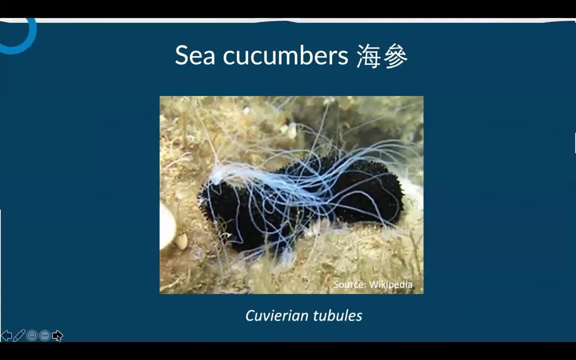 So it's not exactly poisonous, but they do eject this really sticky thread called a cuferin tubules. So they're really sticky and these are their digestive organs. If you mess with them they will stick with you and it's just a pain to get them off. It's not going to kill you, but it's very, very annoying. 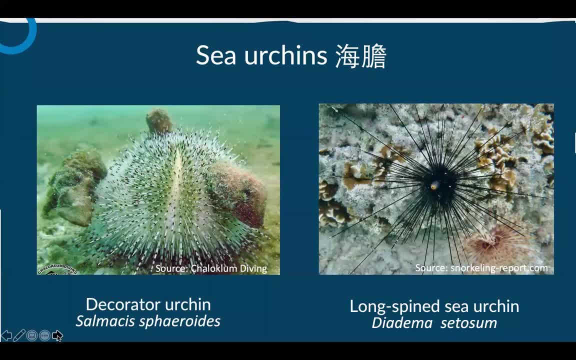 And then we have sea urchins in Hong Kong And many people ask me: can you eat the sea urchins in Hong Kong? My answer is yes, you can eat them, but they're not very tasty, So I'm not. I would not recommend you go and hunt for sea urchins. There are certain things you can hunt which I will tell you. 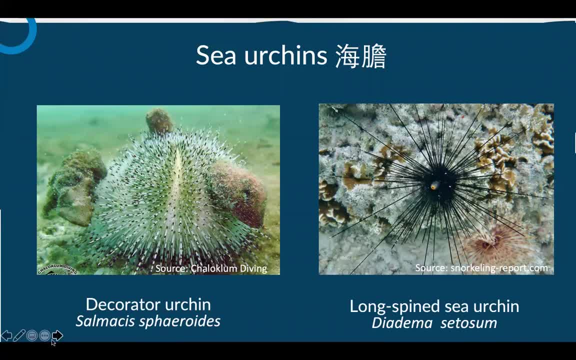 is tasty, but I don't think sea urchins- you should mess with them. So on the left is a decorated urchin and on the right is a long spine sea urchin, which is also pretty common. We have starfish. Starfish are quite common in Hong Kong. 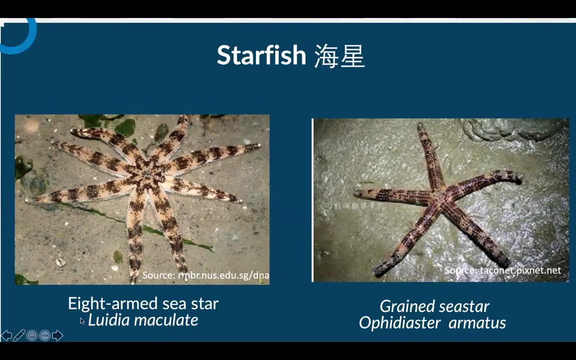 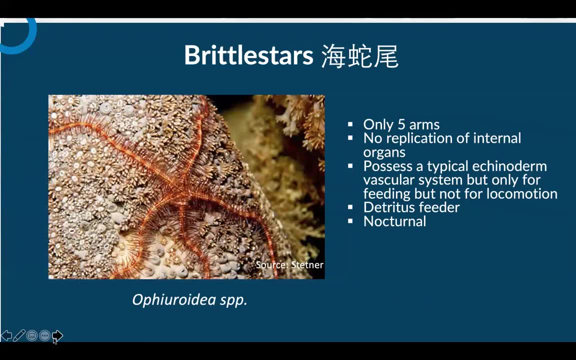 They are not only five arms. some of them are eight arms, some of them are twelve arms, depending on the species- Brittle stars. So they are not sea star. They might look like sea star with five arms, but their arms are extremely brittle and you can come off with it. They are detritus feeder, meaning they eat. 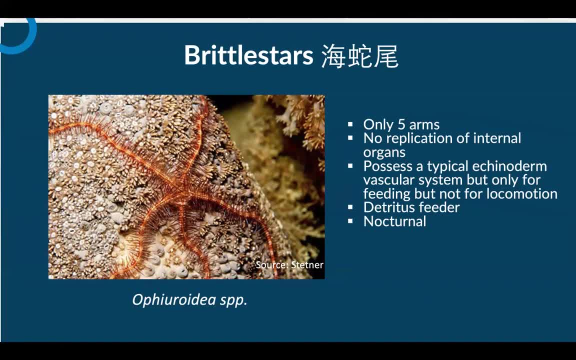 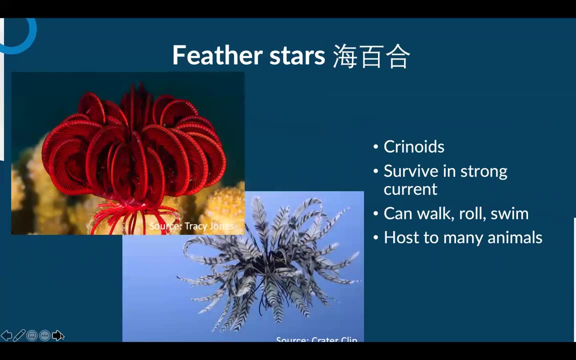 just leftover food in the ocean, whereas sea star, some of them are carnivorous, They eat small animals, They are nocturnal, so in the night time they are very common in the oceans. This is a feather star, Very pretty, very common at the night time and it's very 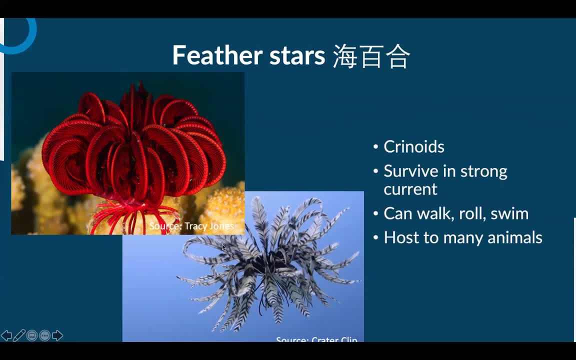 amazing. Actually, the whole thing can come up and actually swim in the water, and they are host to many animals in Hong Kong. They're not extremely common, but they do exist. Okay, now we have another group: that are with many food. 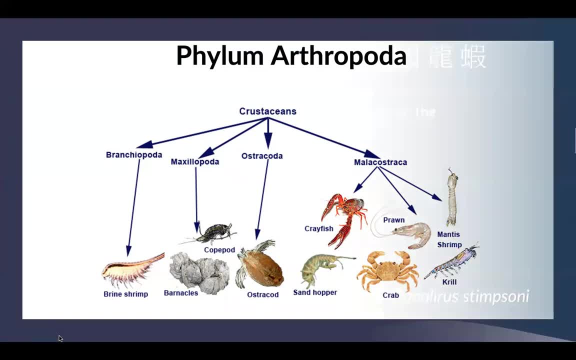 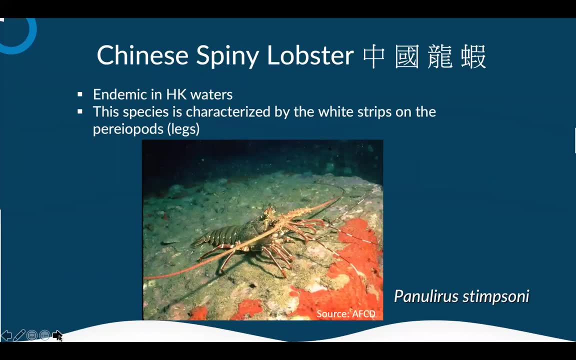 You can see the crayfish, the crabs and all that. So Chinese spiny lobster. They are endemic in Hong Kong water, meaning they are only found in Hong Kong water and not elsewhere. They are very common in the fall, September, October. 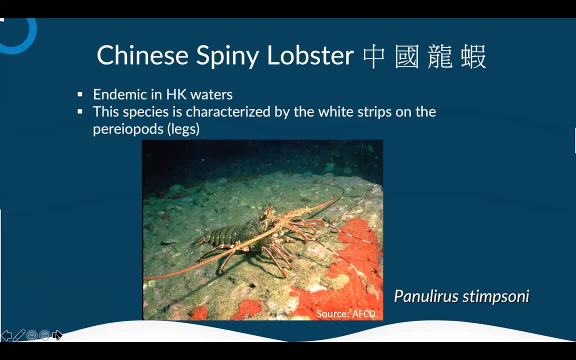 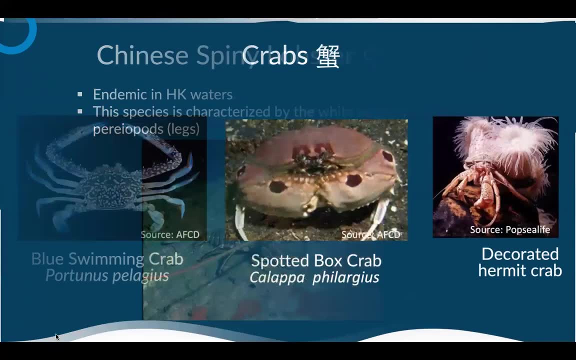 under the rocks. Many people go and fish them, And my advice is: only fish for the bigger size and allow the smaller one to go. Just a different crab. This one is very tasty, so if you are going to eat something, I would recommend this. 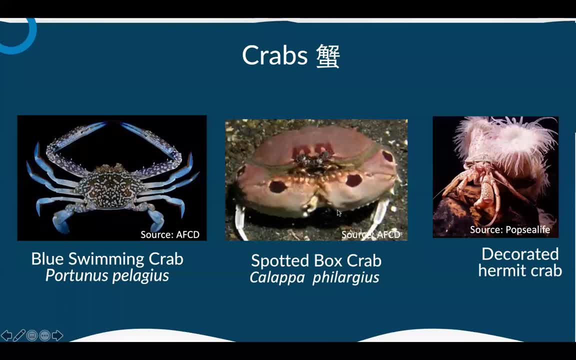 Blue swimming crab is common in Hong Kong. Spotted box crab is less common. Decorated human crab is too small for eat but, as you can see, there's a range of crabs you can find in Hong Kong. We have serums. We have the serums that are big enough for eating. 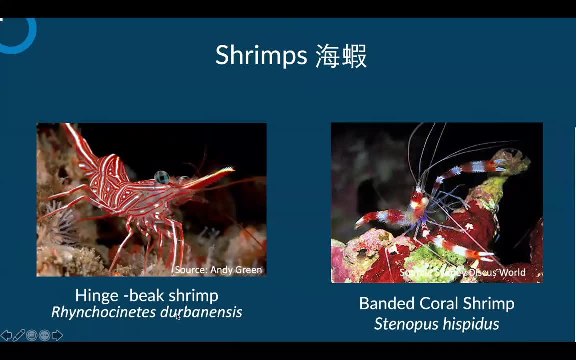 These two are small. These two are very good for thinking. They're usually a found in the bottom of a rock. This is a hingeback shrimp, This is a banded korya and this one is a healthy cod. MS coral shrimp. their body is transparent, very pretty. 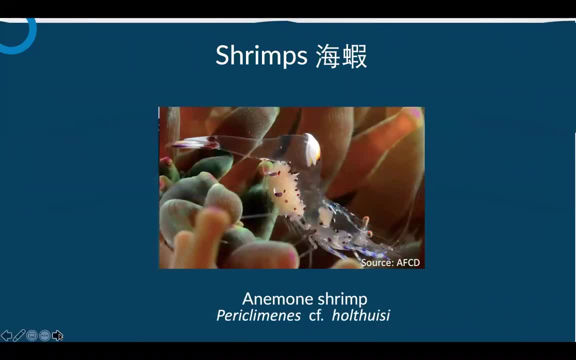 And here's another one. This is an anemone shrimp called paraclaminis. They are found in the anemone, the one with the cat anemone fish, Very, very common, Almost every anemone you find. 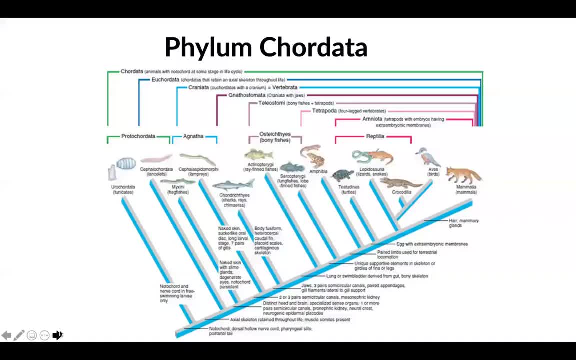 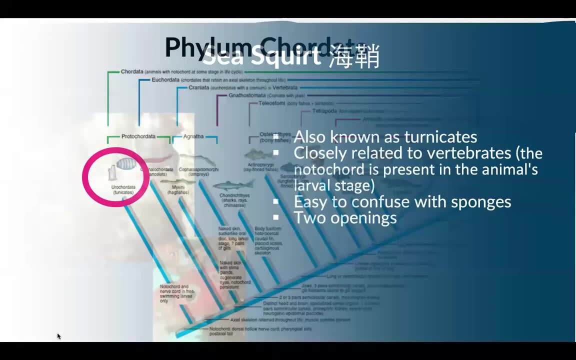 you will find like two or three of these guys Okay. and then we have caudata. we are coming to the end. So they are not exactly vertebrate set, but they have a pseudo backbone. So they have one big and one small opening. 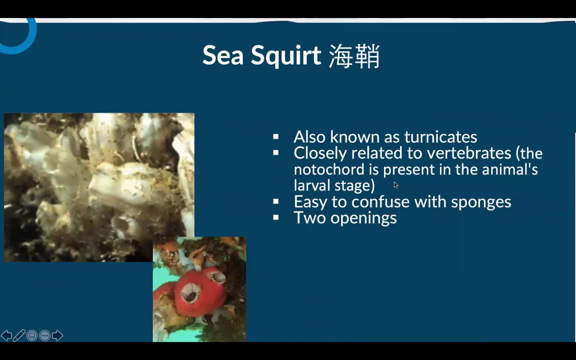 They are closely related to the vertebrates, meaning they have some sort of backbone in the caudanotochord, in the larval stage. They are easy to confirm with sponge, but sponge have many holes. these have two holes only. 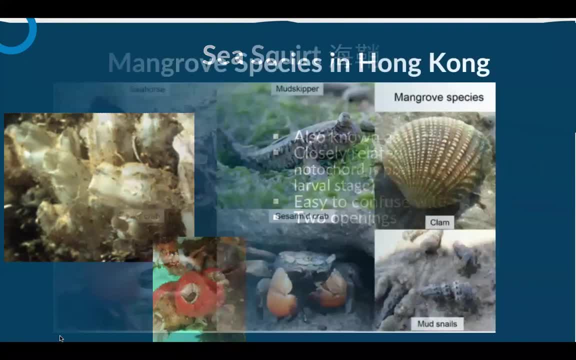 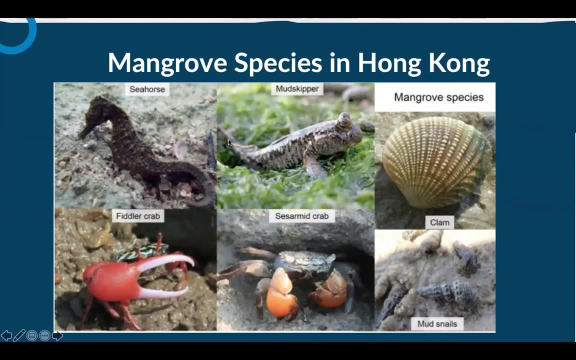 So it's not that hard to tell them apart. We didn't touch in detail but just so you know, we also have different species, different mangrove species in Hong Kong. So we have the musketeer, fiddler crab and all that. 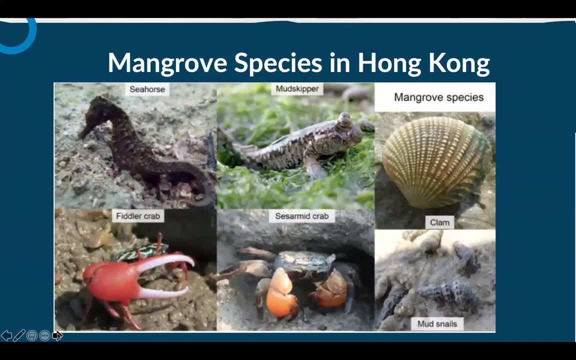 And I would say one of the best mangrove in Hong Kong is in Hoi Ha, if you want to go check it out, Or in Lai Chi Wo. there's also a very good mangrove where you can see these animals. We have four quichua species. 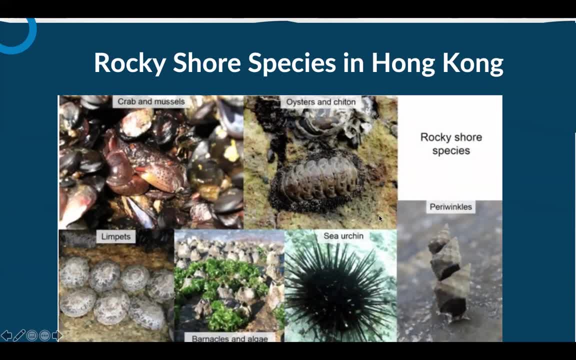 So today I went to Green Egg Island for my own excursion. I find tons of chitons. They are pretty historic animals, just like the horseshoe crab as well, And you see all these limpets as well. Just be careful if you go to Waukesha. 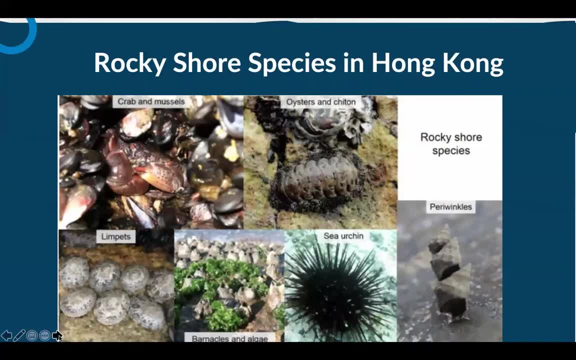 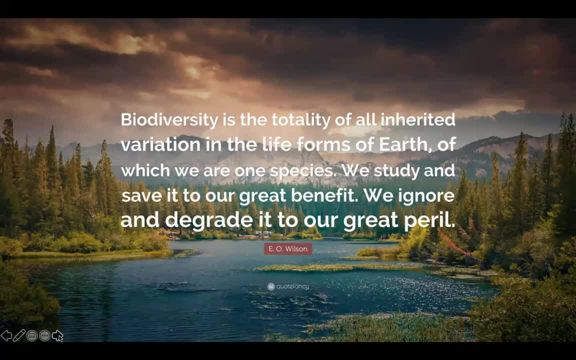 they're usually very slippery. just wear really good shoes to go there. So, yes, so at the last part of the presentation I will tell you a little bit how we might preserve this biodiversity. So in Hong Kong we have something called the BSAP. 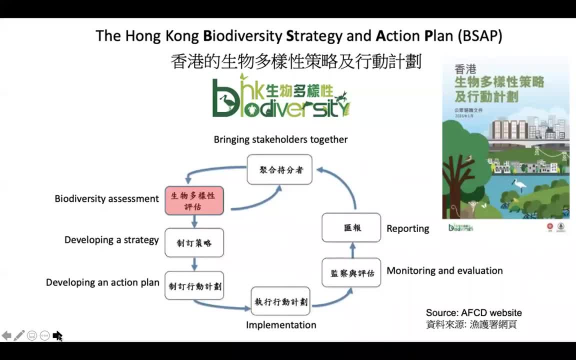 the Biodiversity Strategy and Action Plan. So this is something what the government is doing to bring different stakeholders together to make policy change. But I think today we'll focus on what the individual can do. So, what the individual can do. you might know some of this already. 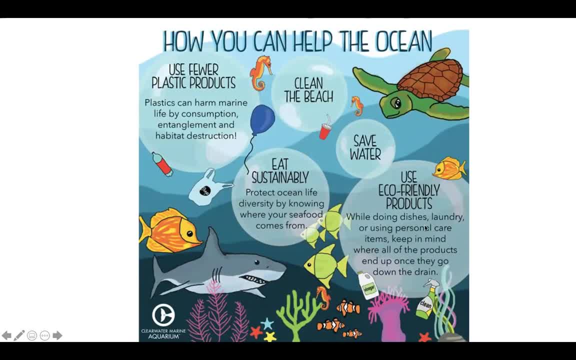 use fewer plastic products. clean the beach. use eco-friendly products. So, for example, if you are going diving or snorkeling, use reef-safe sunscreen, meaning those will not harm the animals. I'm gonna give you a little bit more specific things. 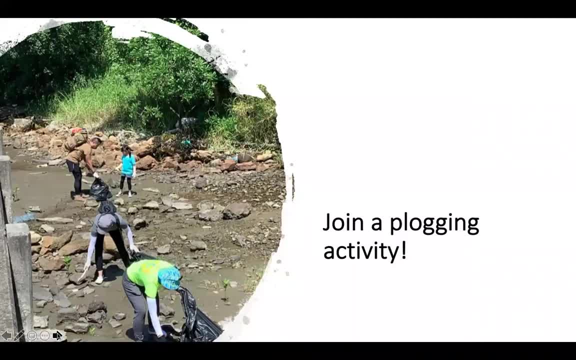 what you can do beyond this. So, for example, if you haven't heard of it, it's called the Pogging, which is jogging and picking up garbage, Eco-marine and Encompass. we sometimes organize this, So if you want to go to a beach and help for cleanup, 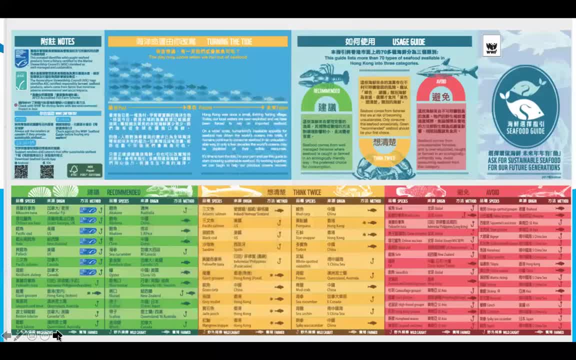 please message one of us. This is also one of my favorite diagram. It's also available in the WWF website, So it tells you which type of seafood is more sustainable. So, for example, a lot of groupers, a lot of the big fish we are talking about. 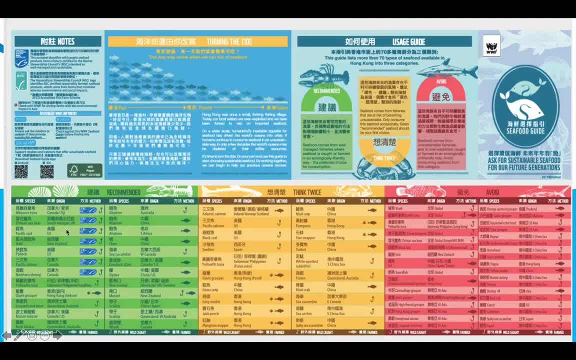 you should avoid them. Some of the fish, like the codfish or the sea bass those are being farmed, is more recommended. So if you are not sure what fish you should order in the restaurant, try to get this diagram and ask the waiter what they're serving you. 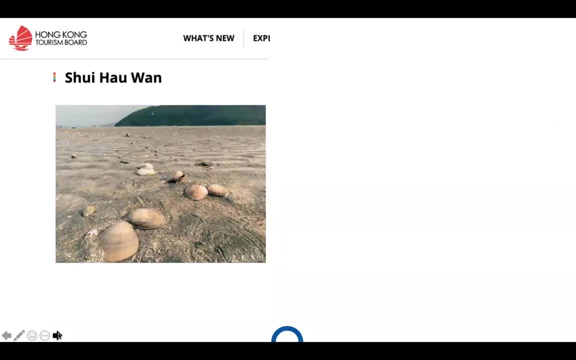 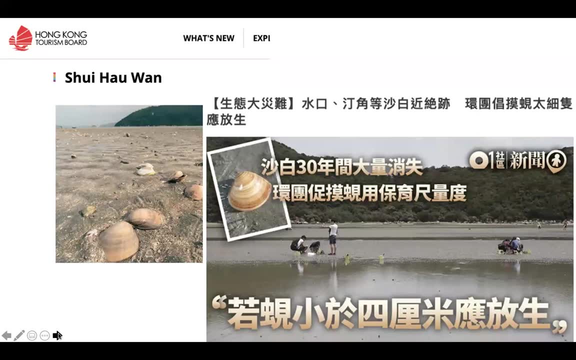 So soy hao wan- I do want to mention this. Soy hao wan has been promoted by the Hong Kong tourism board as a clam digging place. I really not recommend it. The sa ba, which is the clams, has been almost completely wiped out. 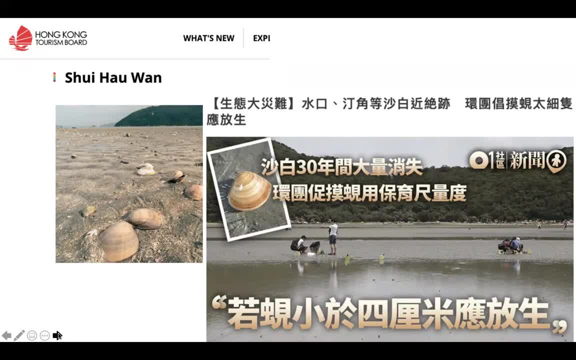 because there are just tons of tourists. Like my friend was telling me, over one weekend there were over a thousand tourists in soy hao And this is also where the horseshoe crab lives, So it's also disrupting the appetite. So there are certain group like the WWF. 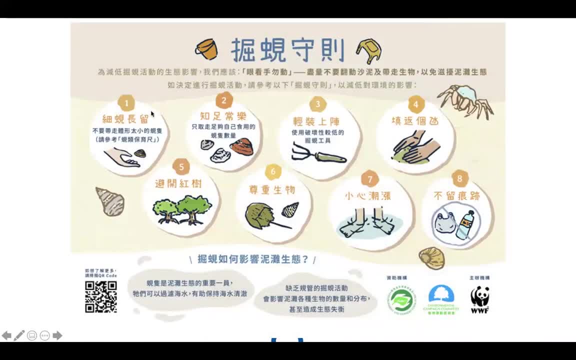 they recommend that you only eat certain size of the crab of the clam And if they are too small, you put it back. My advice is not to get any clams at all. I think if you get any clams it's just going to disrupt the appetite. 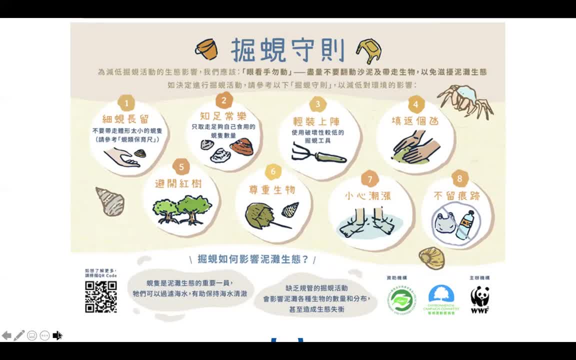 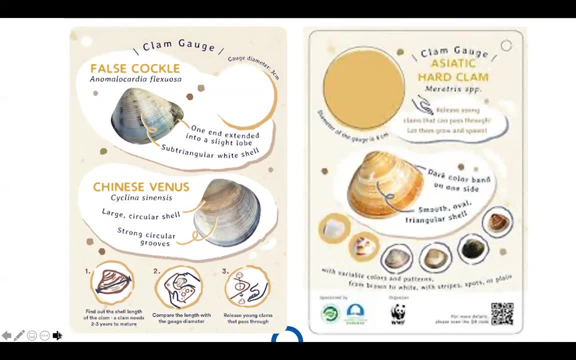 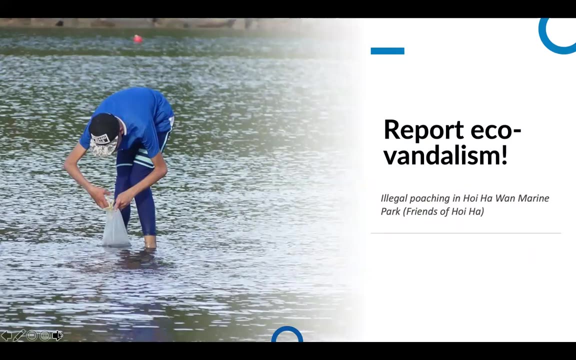 and it's going to endanger them. So my advice is not to do this clam digging thing anymore. So, as you can see, these are some clam gauge that the WWF is doing Again. we put ecofinalism. So, for example, this is a picture I took in hoi hao wan. 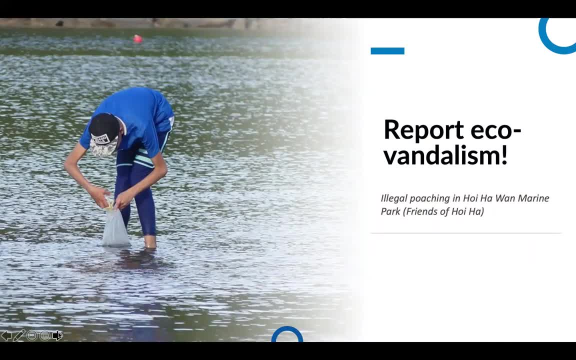 There are some people who are not ignoring the marine park rule and they'll just take whatever they have in the ocean. So you can see this guy it's. you know, it's like getting a sea star away. He's probably making some Chinese medicine soup. 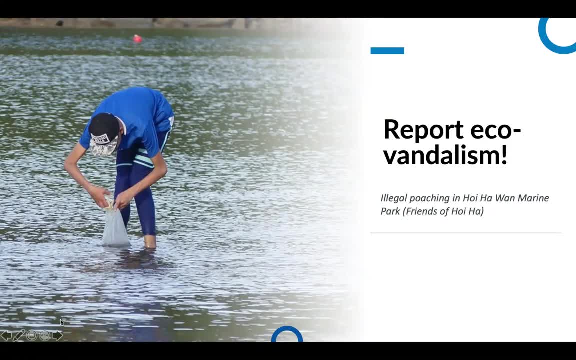 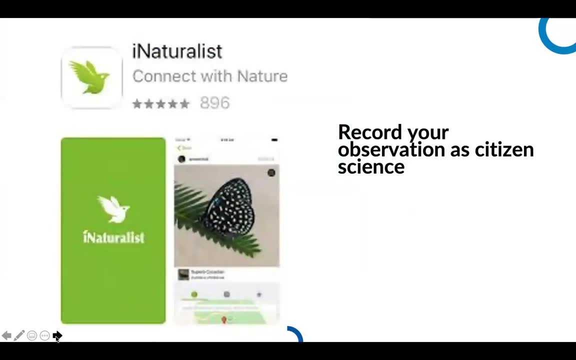 So if you see something like that, report to the authority and try to minimize that. You can also record your observation as a citizen scientist. So if you, if you haven't done this app, this app is both for land and marine species. 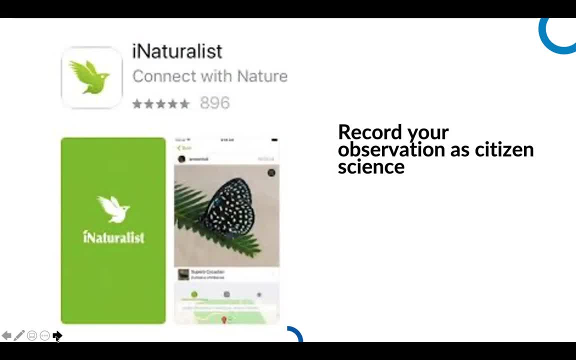 You can record what you see in there, put a picture there and somebody will help ID you. We've got a time and location and you will help uh the uh, the scientists, uh uh, to know more about this animals. 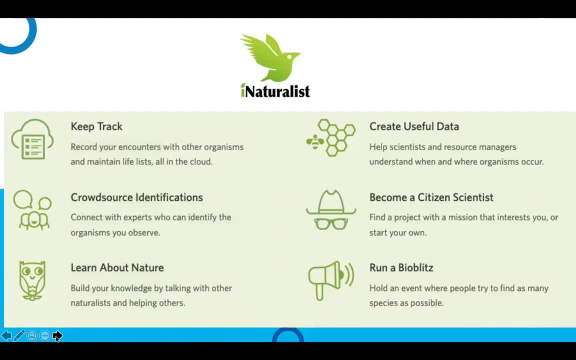 This is some way, uh, uh, the iNaturalist can help. And if you like, uh, if you're like a school teacher or you work in a NGO community, uh, there's a commission called the city nature challenge every year where, uh, in April, where people will compete. 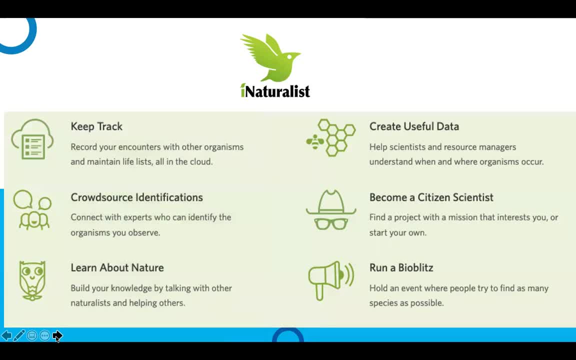 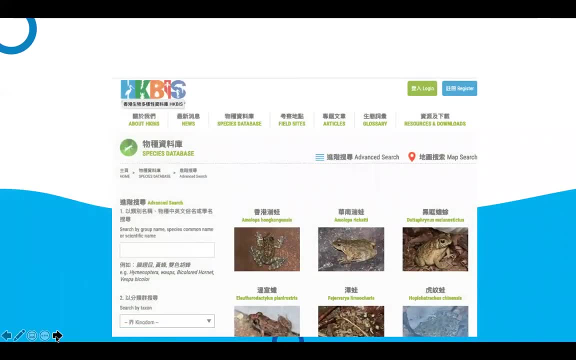 and find the most number of species or the most observation. Uh, and it's a fantastic way for people to learn more about biodiversity. Uh, if you want to learn more about the animals? uh, the Chinese and English name: the hepatite. 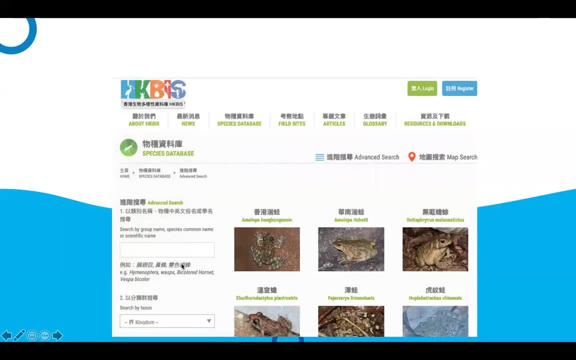 you can go to this website called the Hong Kong BIS. Uh, just type the common name or scientific name and they will show you a picture on where they are. I think learning and awareness is the first type, uh first part for you to better learn about these animals. 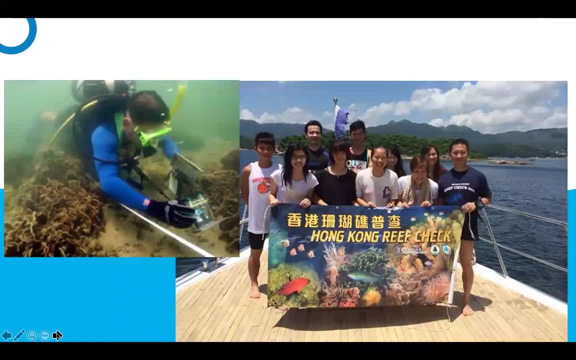 Uh, if you are a diver in uh every, every uh October, November, there's something called a Hong Kong with check You can join and uh, they will, uh, uh, uh, uh, they will do call recording fish recording. 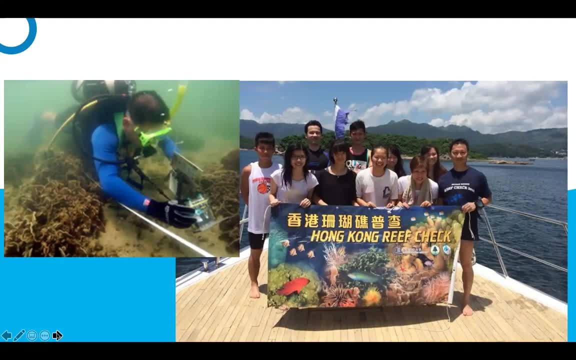 So, uh, it's a way for citizens- for normal, uh uh, regular citizens- to help to uh learn more about the um biodiversity. Uh and uh. so the AFCD each year uh published survey of this results. 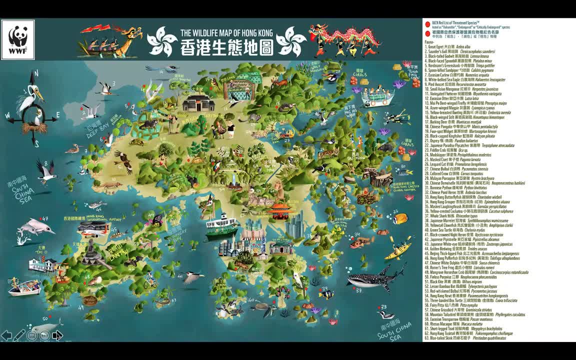 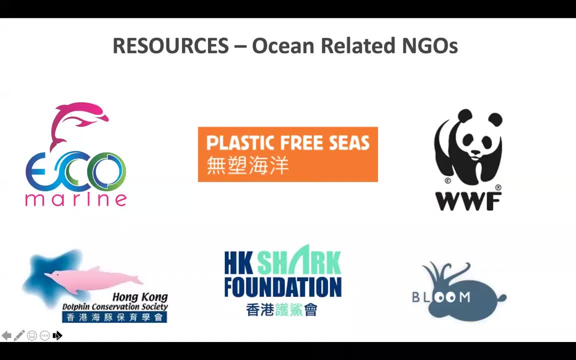 Uh, and if you're interested to know more, this is also available in the WWF. There's a map of everything uh different biodiversity you can find in Hong Kong And if you want to uh, join one of the NGOs. 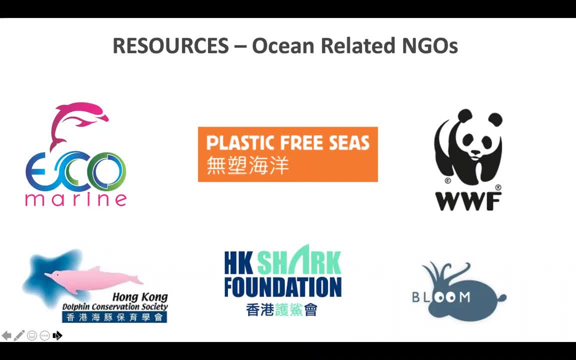 or learn more about the oceans. uh, these are some of the uh uh NGOs uh you can get in touch with. So, for some of the WWF has done some very good work with dolphins and horseshoe crabs and all that. 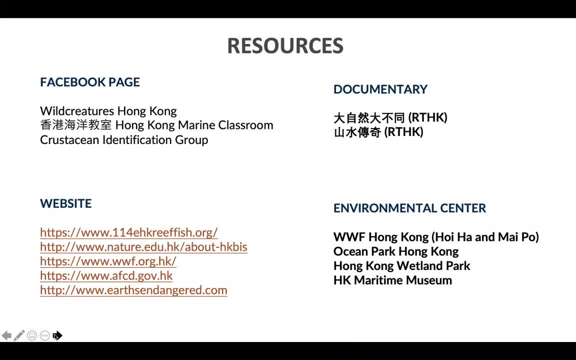 And don't worry about copying this, You will have this site. uh, so just to know, if you want to learn more about the animals, you can go to this websites. And, uh, these are some really good documentaries on the Hong Kong biodiversity as well. 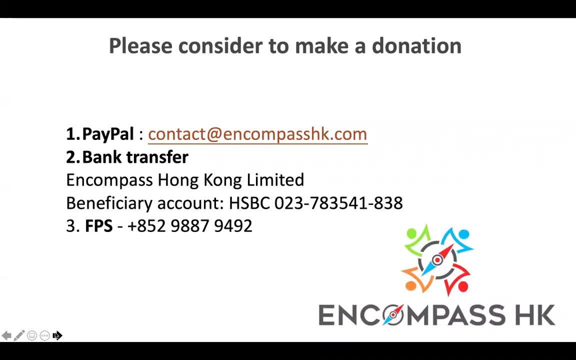 If you like us, if you like Encompass, if you will consider to support us, uh, so we're doing this for free. If you want to support us, uh, please, uh, donate to us at one of this method. 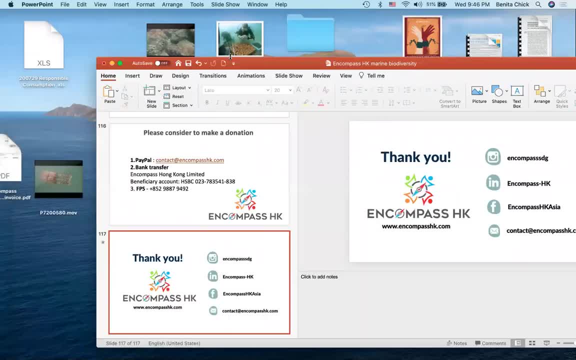 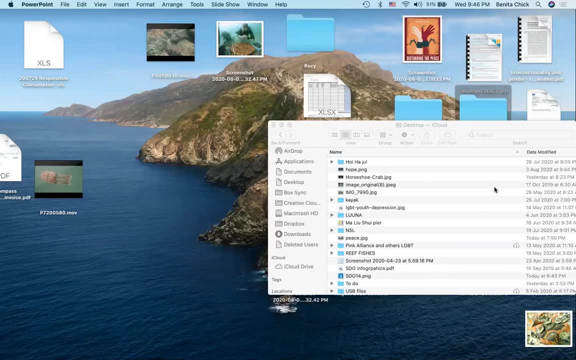 And yes, uh, I think I'm on time. We still have 15 minutes, Uh. so, yes, uh, maybe now is a time, uh, you can ask some questions. Yes, Uh, so Alexan Alejandra was asking, uh. 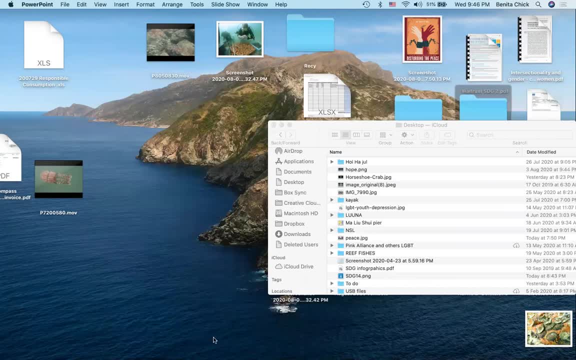 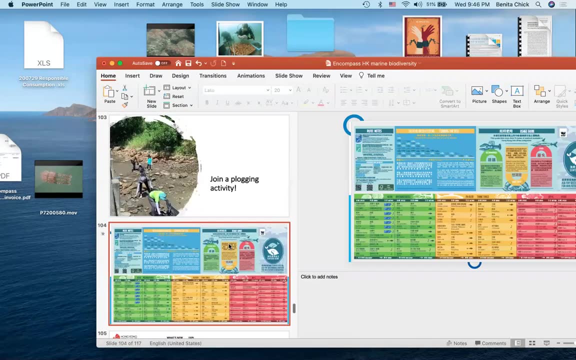 which fish are advisable, Which fish are advisable to eat. So, uh, like, uh, what I said in the uh the presentation, uh, let me show you again. So I think this is a good slide. Uh, I will share with you this, uh. 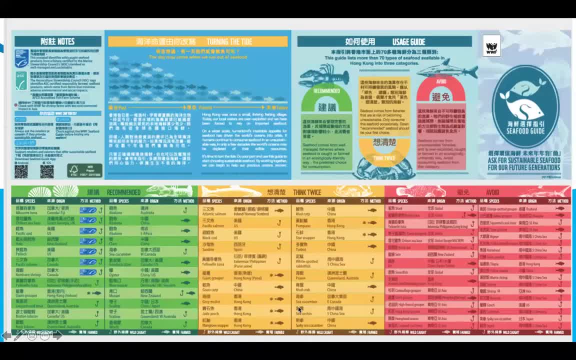 this presentation there, uh, uh later. So these are the recommendable. Uh, what sea snakes are there in Hong Kong? Uh, yes, there are one or two species of sea snakes. I don't exactly remember what are them. uh, 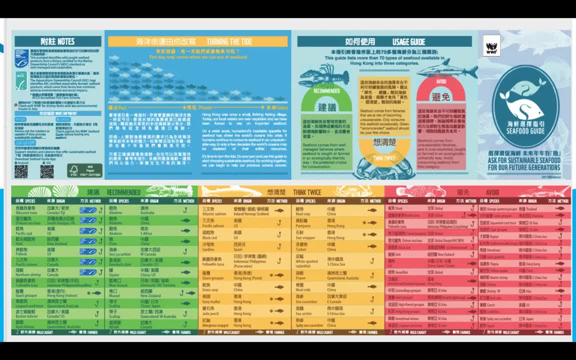 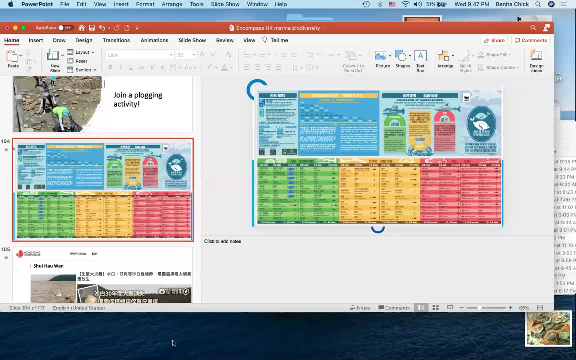 but I would say they are not common in Hong Kong. The eels are common. uh, sea snakes are not that common, Yeah, Any other questions? What is your view on a dolphin who come to live with deep water bay earlier this year? 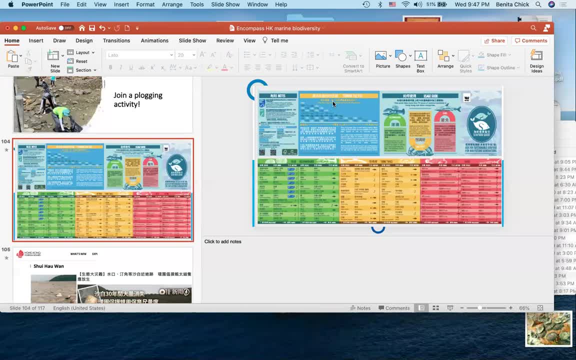 Uh, I, I think the uh I, I, uh, I, I, I, I, I think, because of the habitat destruction, that the dolphins are losing their appetite, so they are just going anywhere they can find. so it's definitely not normal that they are going out of their usual range, but I 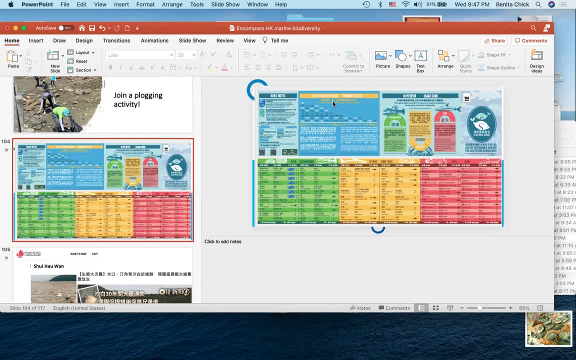 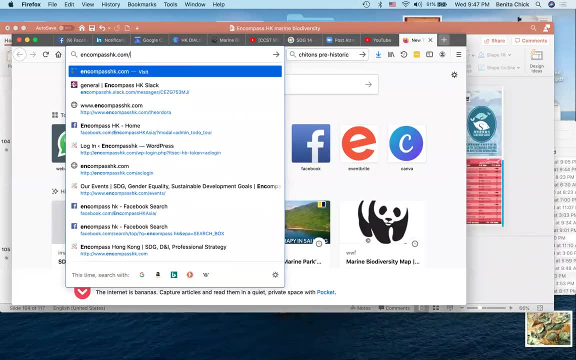 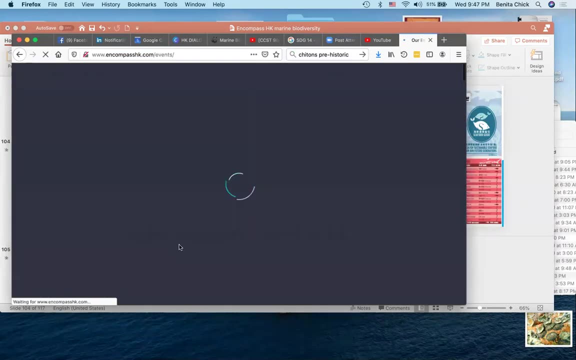 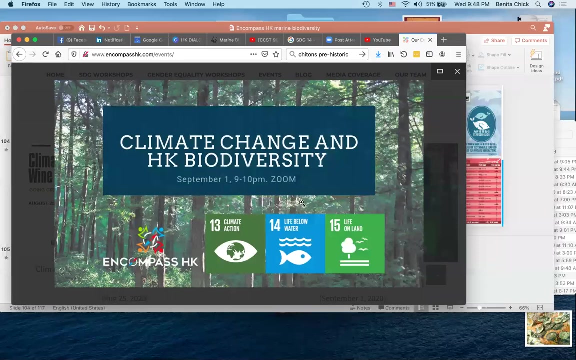 think that is happening with a lot of different species and- and if you are interested, I'm doing a talk later on this this year, later this month. let me show you, yep, so we'll be doing a talk on climate change and Hong Kong biodiversity. so the dolphin is not exactly climate change, but I think it's. 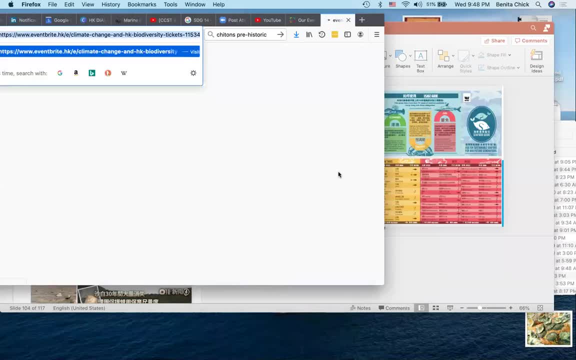 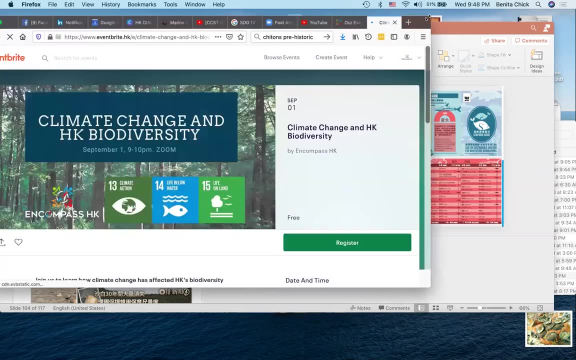 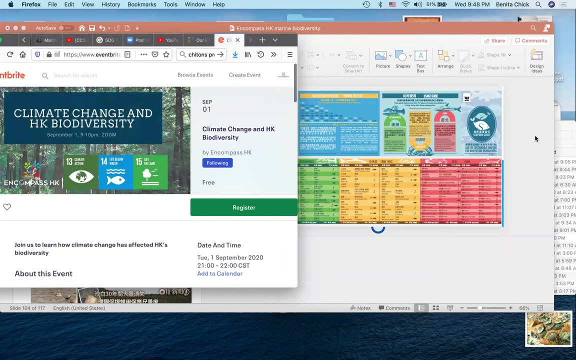 more habitat destruction, but if you want to learn more about animals and why some of them might go to different areas, yeah, this talk will address that. let me unmute you guys. I will send you the PowerPoint after today, so don't worry, I'll send to you by email, and also the recording as well. so any questions? 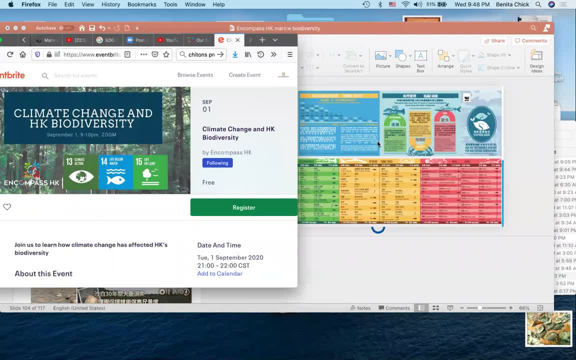 sorry, I know I go very fast, but I just want to make sure I go for the content. yeah, so it's by no means a full comprehensive of what else die in Hong Kong, but I hope to show you some species. are there any organizations or is government doing something to find a pine? dolphins- a new 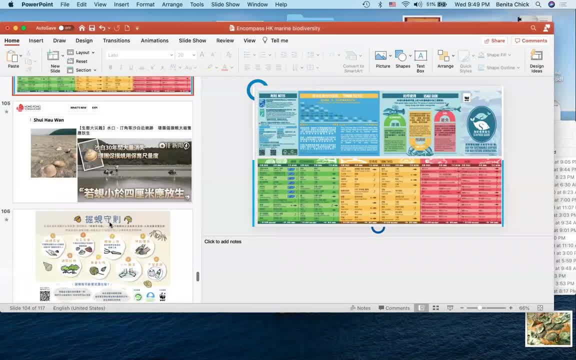 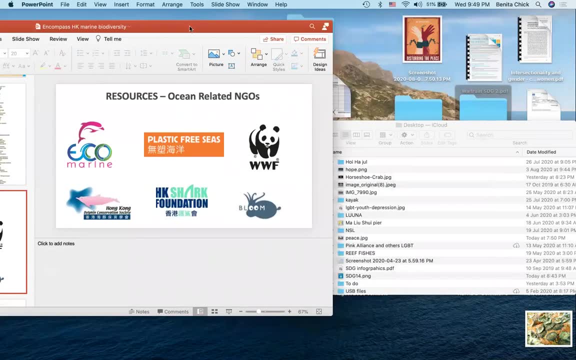 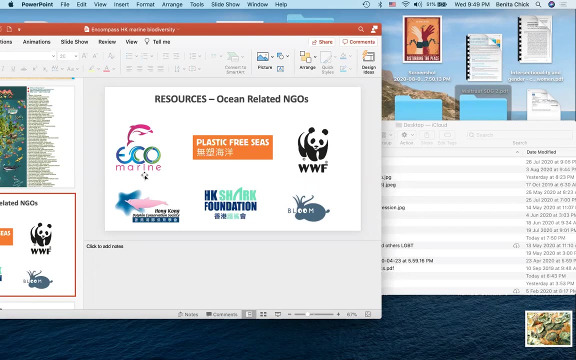 room, I think, the Hong Kong Dolphin, this one, the Hong Kong Dolphin Society. they are trying to work with the government on the best way to conserve the government, the habitat. oh, I forgot one one here as well: the OPCF Ocean Park Conservation Foundation. they also did a fantastic job in, in, in. 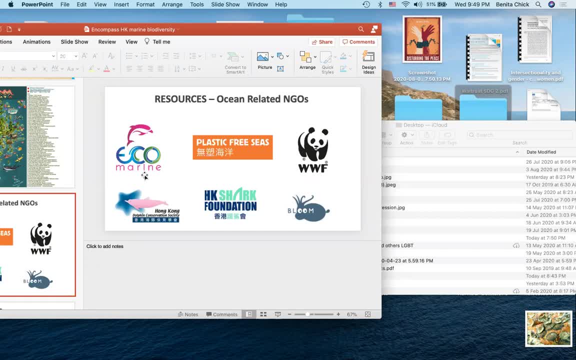 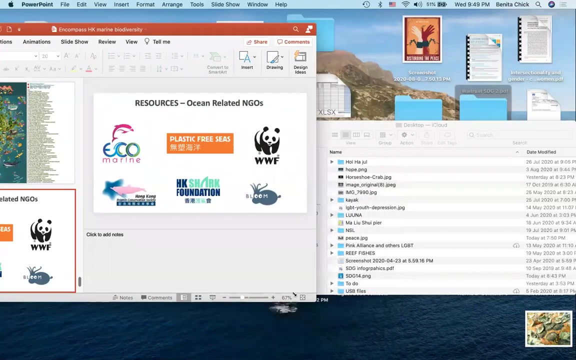 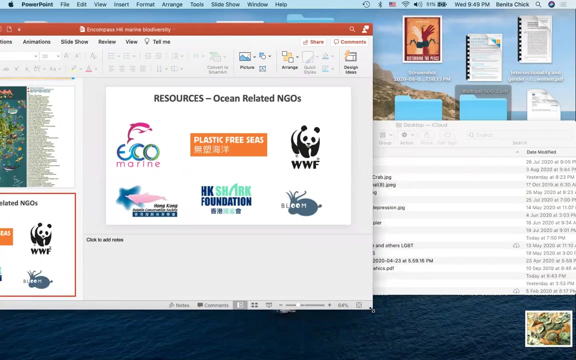 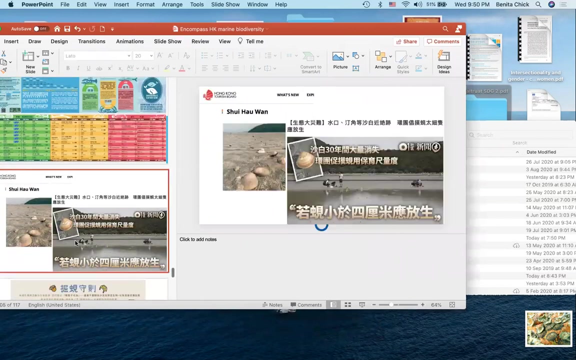 the dolphin research. so, yeah, I really I don't know. where do you guys live? are you guys from Hong Kong, are you from somewhere else? but go to Hawaii or don't think so how? the place where I imagine the clams, like I was there. I was there two weeks. 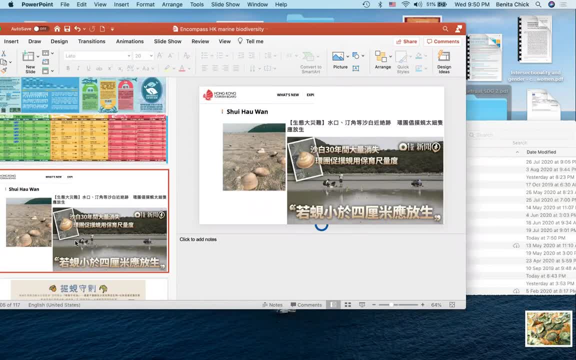 ago and there were like a lot of sandy shore animals, different snails, really pretty. just just be where where you walk. you don't want to walk on horseshoe crab, but it was quite difficult for me. I was, I think I spent an hour and a half and I. 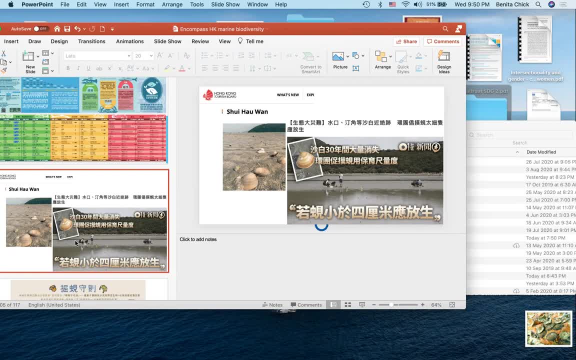 only find one. yeah, I think I spent an hour and a half and I only find one. she was like, oh, I didn't even catch anything. she was like, oh, I don't know what that is, and I thought I was going to go get it. she said, no, okay, so here I go. here's the next, the next thing. I was like, oh, oh, I think this is the without out of this. I'm just going to let you guys know what I do. but I was like: how do we think about these things? because I'm gonna talk to you. do we're gonna talk to you about how? 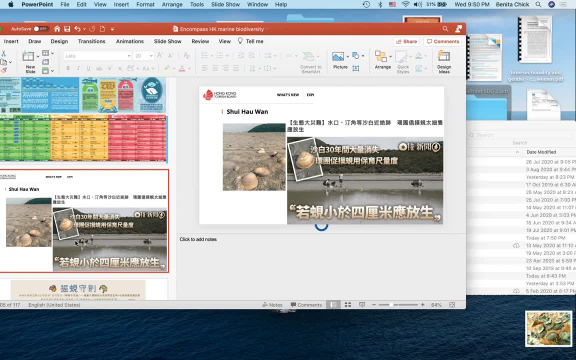 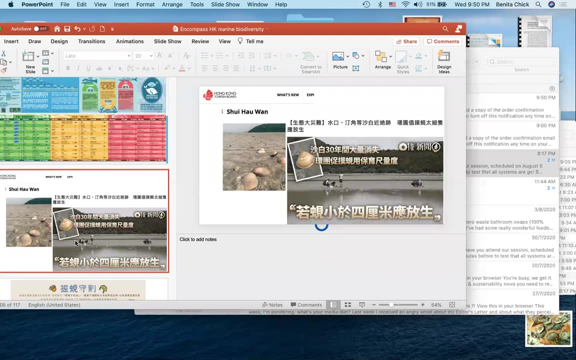 and if you are interested in diving or snorkeling or learning more about the hepatite, you can message us on Facebook or email. hopefully, after this covert is over, we can all go and explore Hong Kong a bit. where is the best place to learn or observe biodiversity in Hong Kong? I mean to learn? there's a marine. 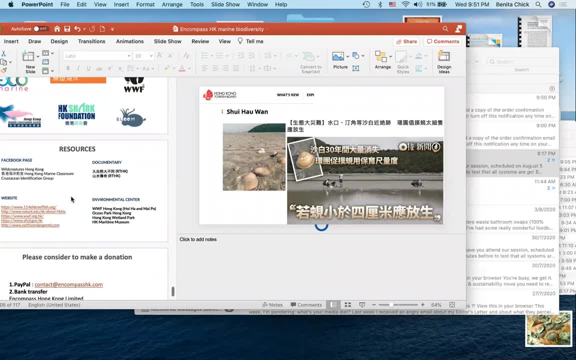 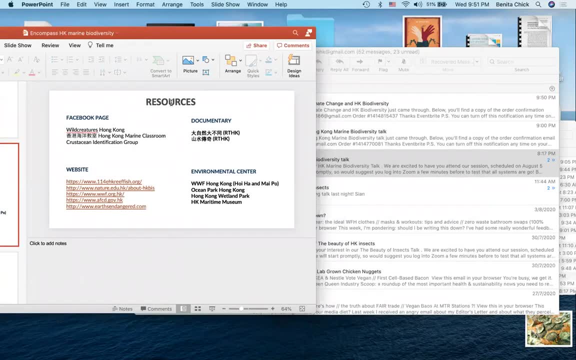 biodiversity I would. I mean it depends on what kind marine biodiversity is quite, quite a big. I mean some. some people are specialized in dolphins, some people are specialized in crabs. I would like, if you want, to observe the WWF. the Hoi Ha Center is quite good, the Hoi Ha Center have have a glass bottom boat. you can. 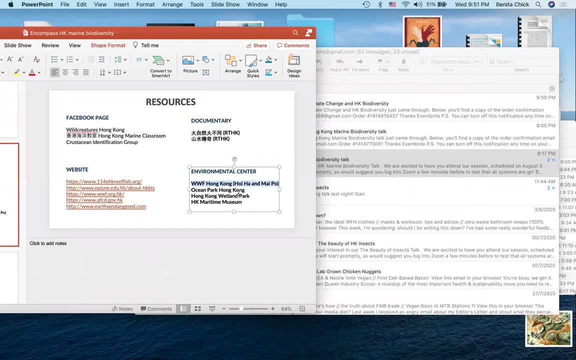 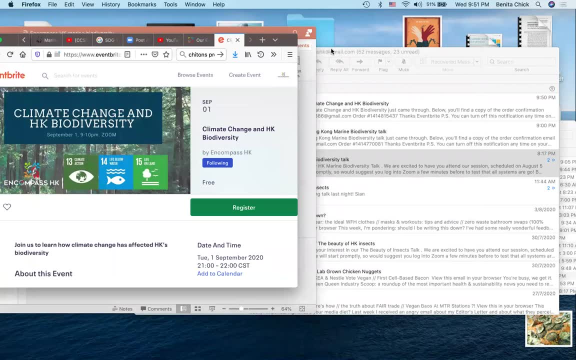 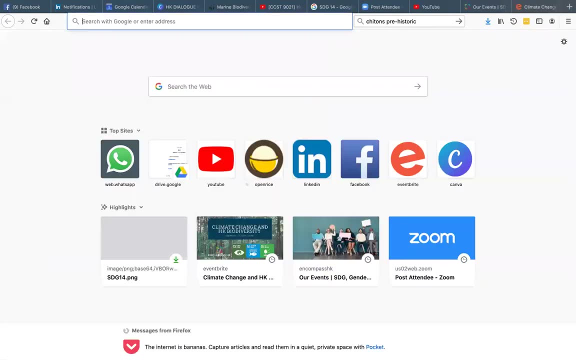 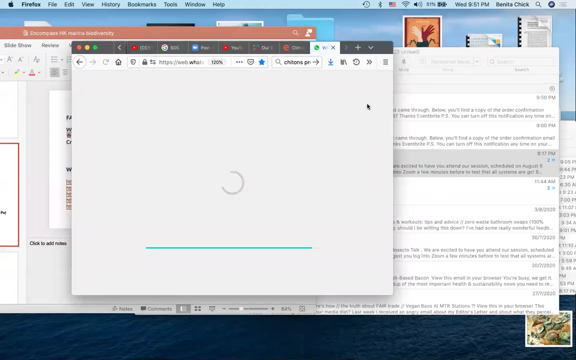 all learn about the different animals and they explain to it to learn. I think there are some. let me show you there. there are some companies in Hong Kong. they teach the marine eco tourism class, where they teach you different animals in depth. but a lot of that, a lot of. 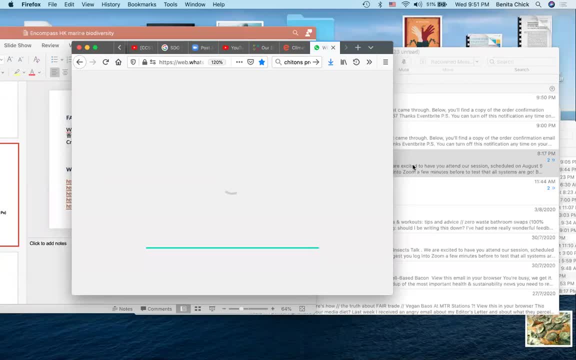 those are in Chinese only, so I don't know if you're English speaker. they're not that. unfortunately, I think, if you are not in a university, there are not that many resource where you can learn marine stuff online or in person. but there are some really good books by 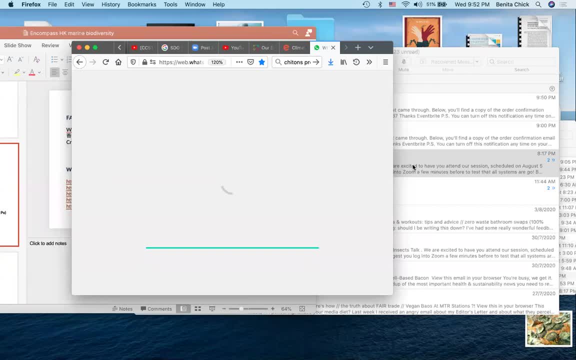 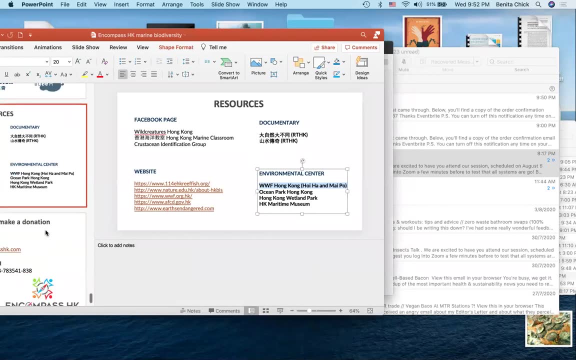 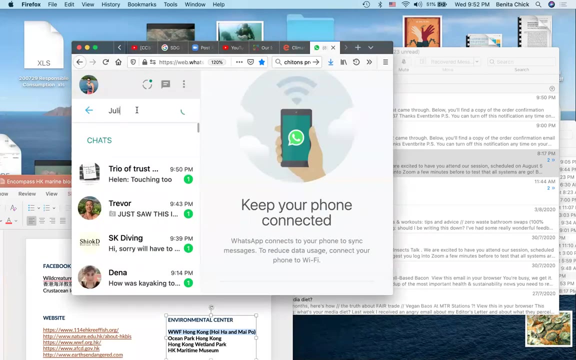 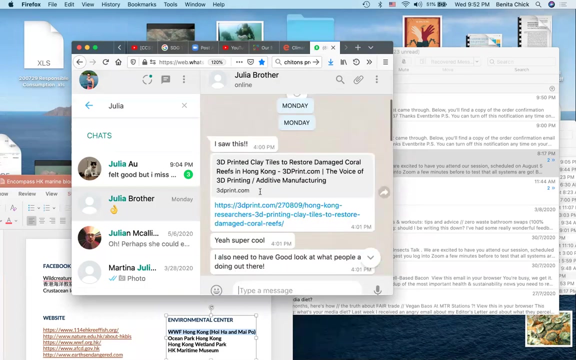 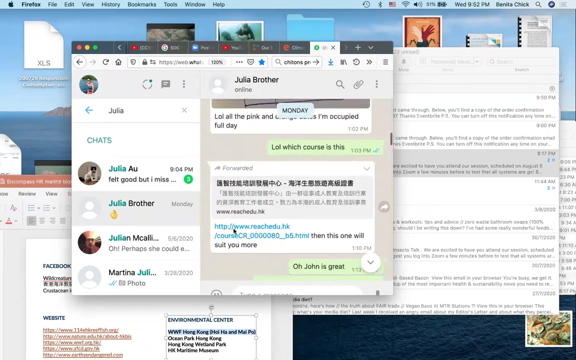 the AFCD out there on the marine biodiversity: more resource to learn about marine science. wow, that's a that's a very big topic. let me. let me show you this one first. okay, you. so this is for Alejandra, and she mean him. this is a company in Hong Kong that 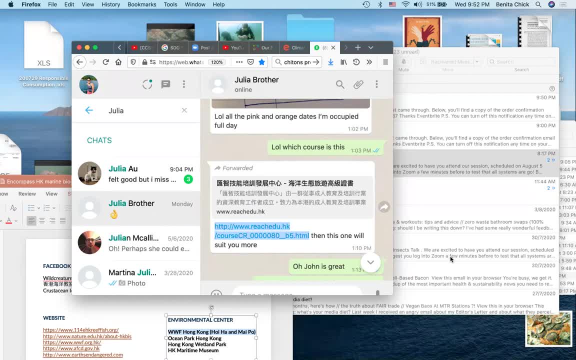 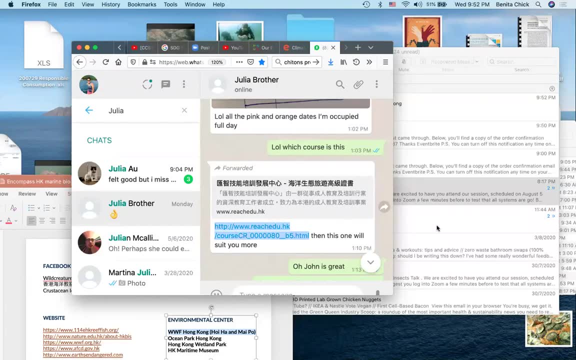 they do marine biodiversity courses and she said she might go to the Arctic, so if you're interested- I think it's in Chinese only, if I'm correct- so yes, more resources to learn about marine science or biology. I mean, NatGeo have some really good videos as well. 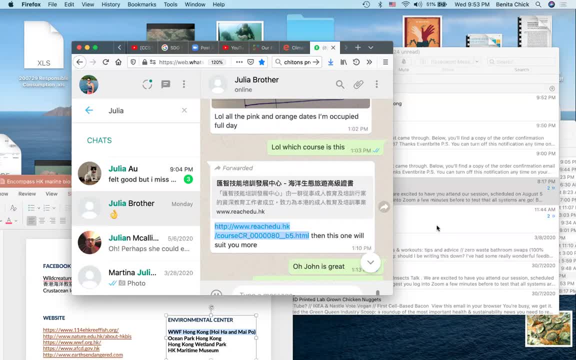 if you want to learn marine science, I can recommend some books. maybe I'll put that in the summary email. how do you propose a balance between heritage, eating shark, fin, turtle shell soup, drinking horseshoe crab blood and conservation? I think I mean, if you ask me, I would say: 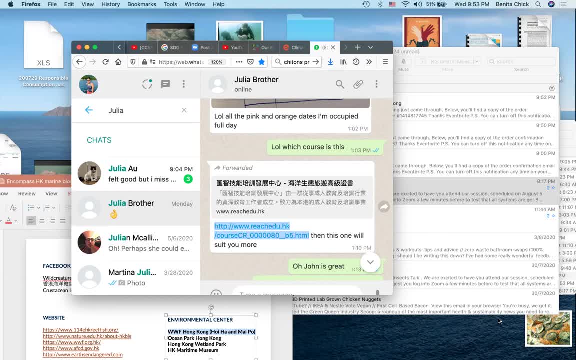 don't do any of that. don't eat shark fin, don't eat turtle shell soup, don't drink horseshoe crab blood. but I understand, sometimes you need a compromise because, like the camps, WWF is telling people to only catch a certain size and not asking. 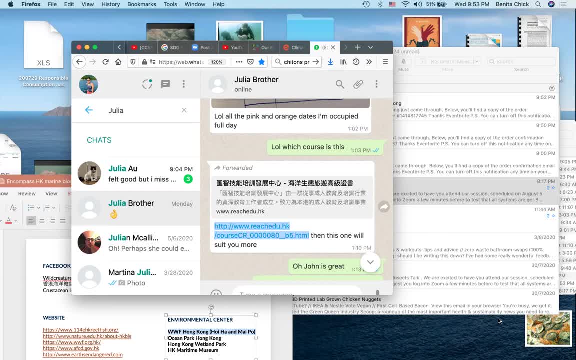 to not catch at all. so I think they realize it's impossible to tell people not to fish at all, but rather than to tell them to just fish for a certain size. so yeah, it's always a dilemma. I think some people are really stubborn in their way in the fishing. 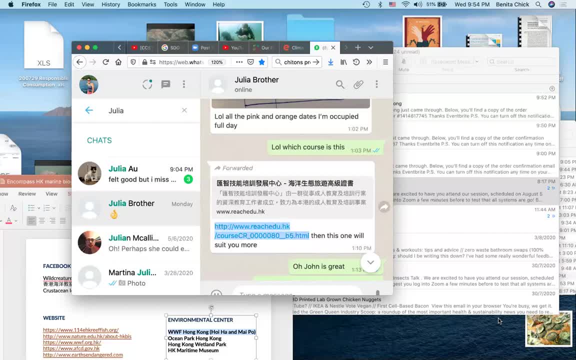 so I think to go from 1 to 0 is difficult, but if you just ask them for a certain size, it might be easier. I mean, as I said in the beginning of the presentation, I think the Hong Kong marine environment did improve in the last few years. 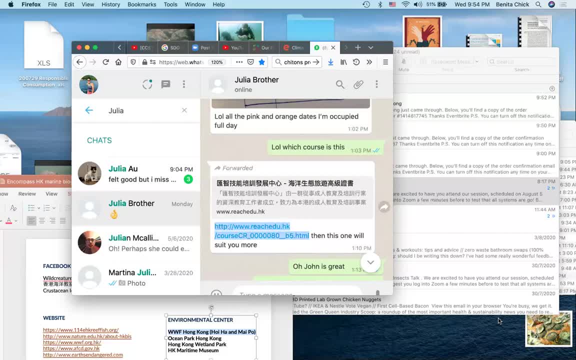 I think that has a lot to do with the fishing ban, with the government saying certain amounts you cannot fish. do fishing? it does make a difference. so, yes, it's always a dilemma, and that's that's a dilemma not only in marine biodiversity, that's also in like buildings and everything. 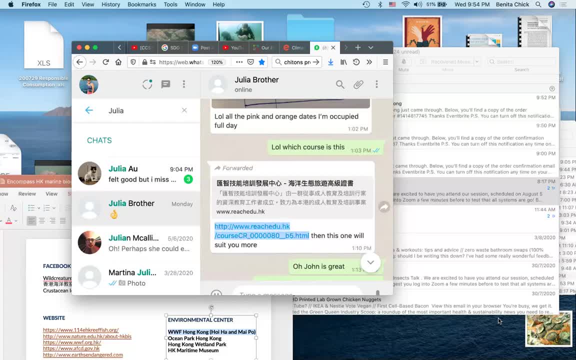 or culture. how do you preserve something while there's new things happening? yeah, I think there's a lot of different things that need to be done, and I think the most important thing is not to let the environment be the only place you can do it, but to keep it there. 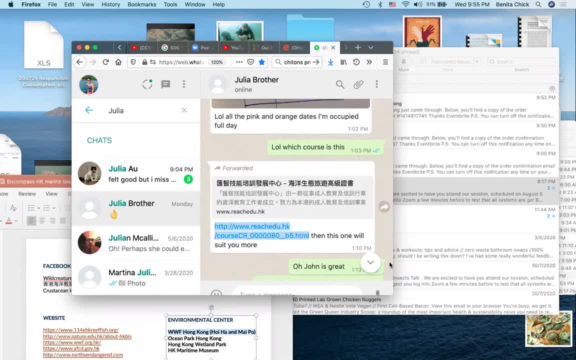 and you have to keep it there. it's really important, because if you can't keep it there, you can't preserve it and it's not really worth it. because it's not worth it when you have to change your heritage and you have to do it yourself. 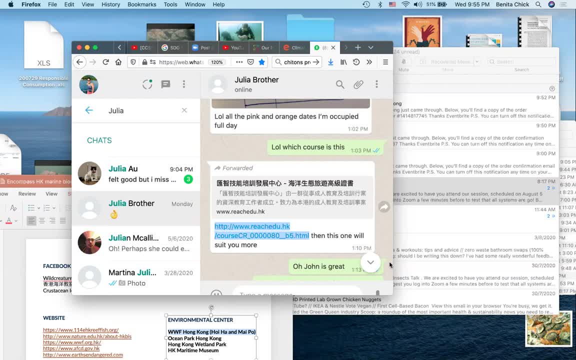 it's not a good thing, and tell them about the wonderful animals we have in Hong Kong. As I show you, we have some small invertebrates. it's really diverse. So thank you everybody. so have a good night. have a good night everybody. Captions by GetTranscribedcom. 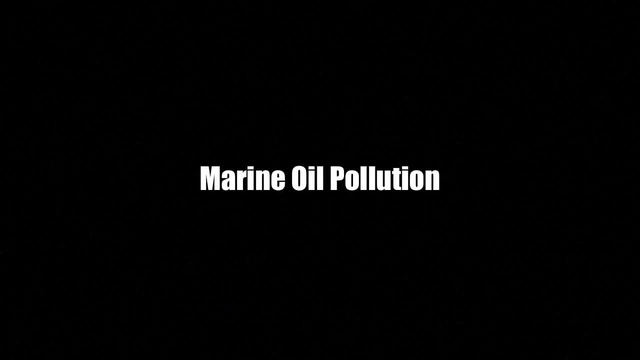 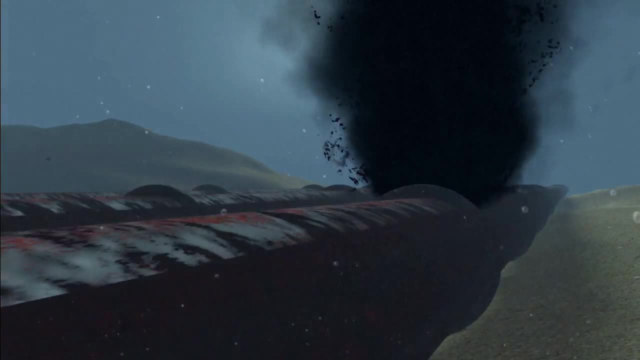 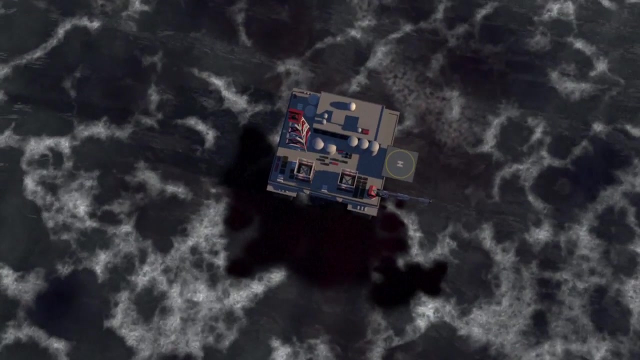 Oil pollution in the oceans can have a disastrous effect on marine life. It often takes a major incident at sea, like a tanker spill or oil rig explosion, for most people to grasp the extent of the problem. Oil slicks can drift towards coastlines, killing seabirds and marine